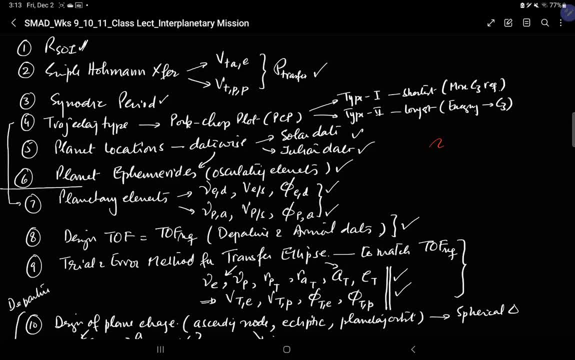 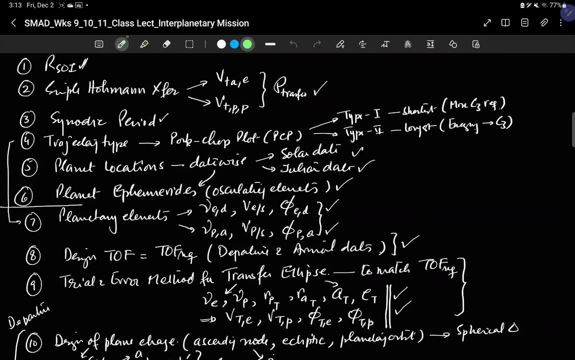 To this point what we have done. I am just going to quickly repeat those items. We have finished this point: the calculations of the sphere of influence. then we started off with the basic and a very simplified calculations which was related to the simple off-min transfer which was from the ideal location which is actually the two planetary positions lying at opposite fc's. 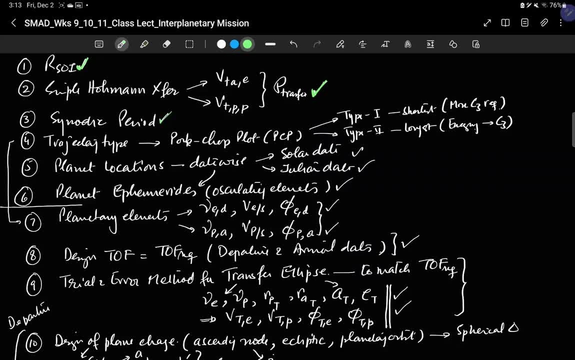 And then we calculated the sphere of influence. We did the synodic periods for different planetary bodies. Thereafter we went for the trajectory calculations, and the trajectory calculations led to the development of the PC plot, which is the, and this was able to give us the value of the C3 and the variation of our type 1 and type 2.. 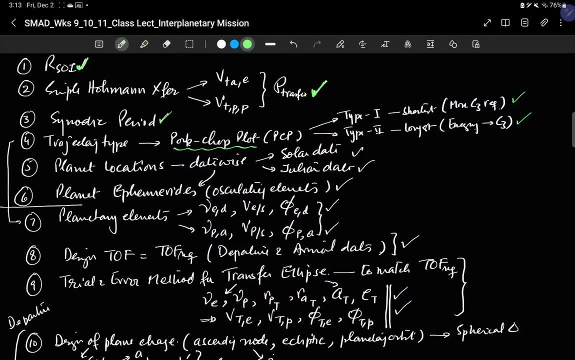 And there was a lot of mathematical model that ultimately culminated into this, the Pokchop plot. After that, there was Okay to do this thing. we had to first develop the position of the planets according to the solar dates as well as the Julian dates, and then, from there onwards, we used the ephemerides services of JPL, for example, to calculate, to determine the ephemerides of the planets on the dates of departure and arrival. 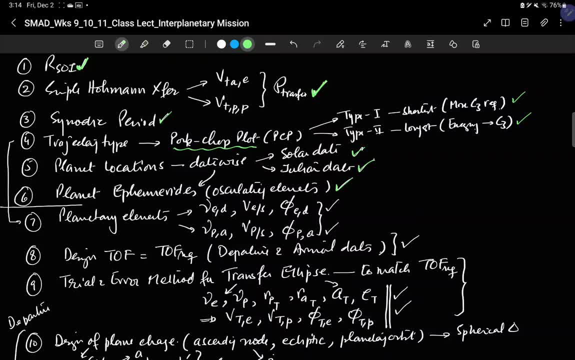 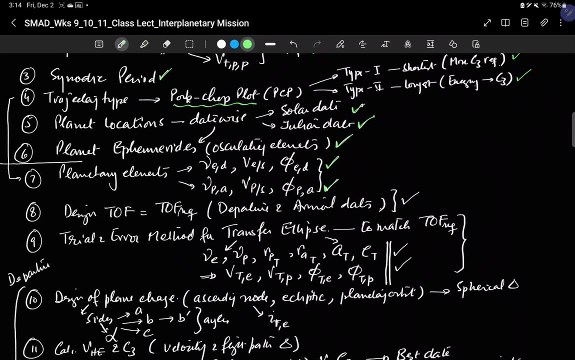 This was all done to basically start the calculation for the PC plots And then, once that was done, after that We did the planetary elements calculation, completed the planetary orbital elements calculation, which was the true anomaly and the velocity and the and the flight path angle of the, of the of the planet at the departure and that of the arrival. 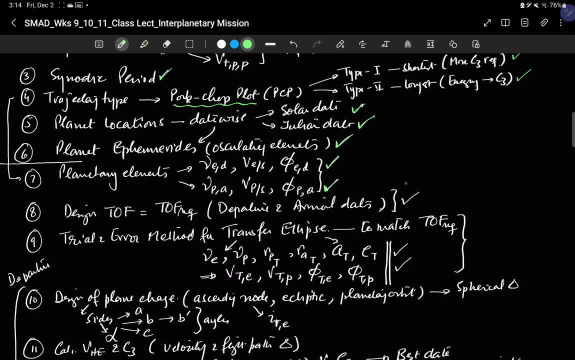 Once we had the time of flight, determined from the, from the difference between the, the travel time, between the departure date and the arrival date, So then we carried out a trial and error method. The trial and error method was to fit the, the, 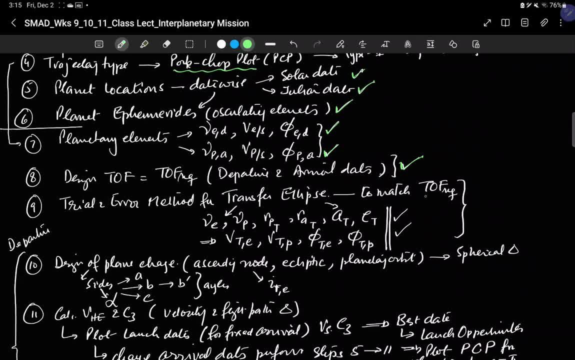 Transfer ellipse such that it would have the, it would meet the requirement of the TOF required, which was the time of flight between the between the departure of from the from one planet and arrival at the other planet at the center sphere of influences. 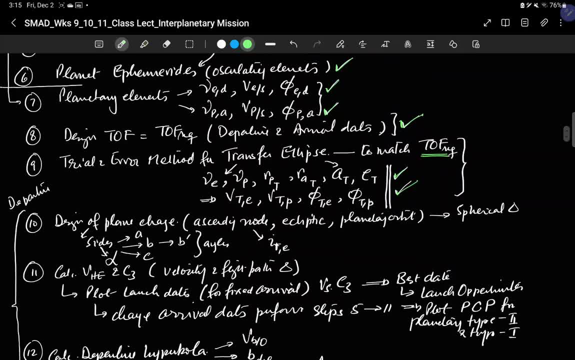 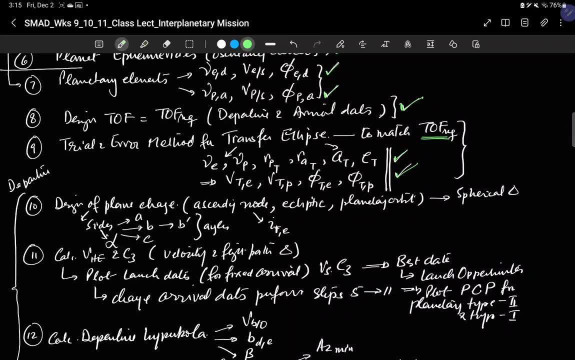 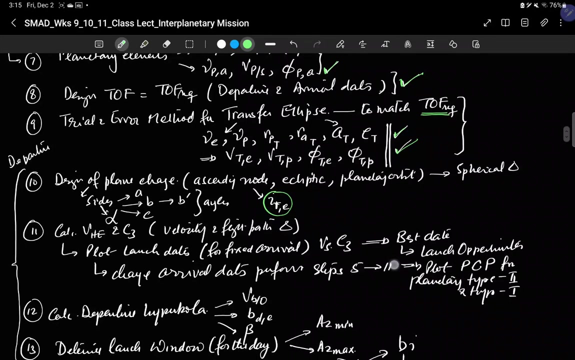 So this calculation was done And then we did the departure trajectory in the in the last lectures and in which we did the, the design of the plane change, The plane change that was give us the, The, a spherical triangle, and the spherical triangle then would help us solve for the, the inclination that was required from the, from the earth on its, on its transfer to the transfer ellipse and to get into that transfer. 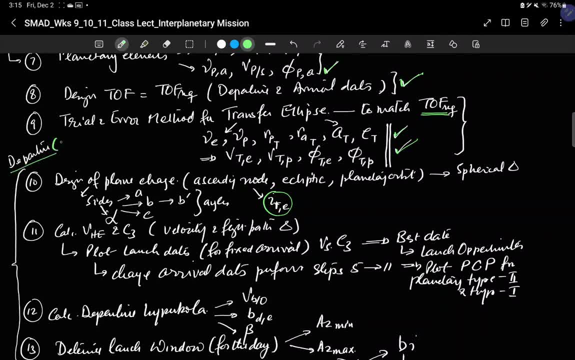 This is now the. this solution was being solved inside the sphere of influence, So we were inside the RSOI and which was actually a hyperbolic Trajectory calculation. So all these were performed and it was the most important thing was the calculation of the hyperbolic excess velocity, the VHE excess velocity and the third cosmic energy. 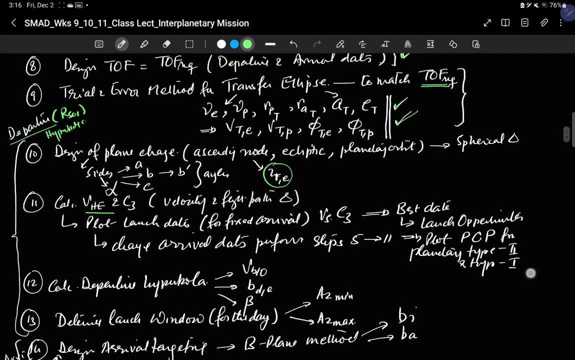 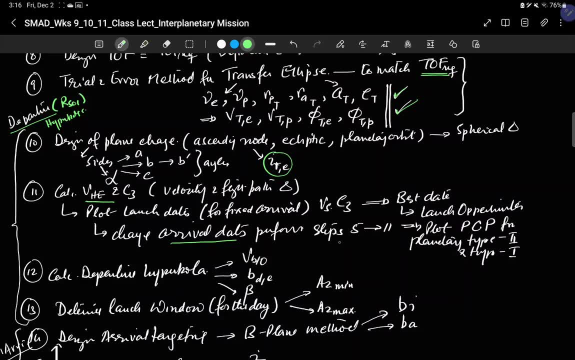 And then we were able to calculate, based on this, the check for the matching of the arrival dates on the on the chop plots, and see if we were able to match the same. The results were matching with the chop plots data for the type one. 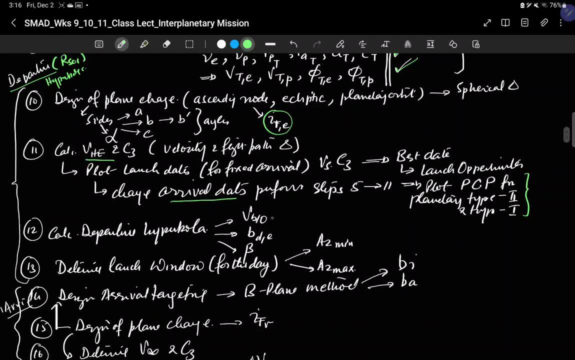 Our type of that You would ever was applicable. We also got really the burn out velocity Are the. We also determined the science of the, of the hyperbolic, the orbit, as well as the, the angle of the change of the. 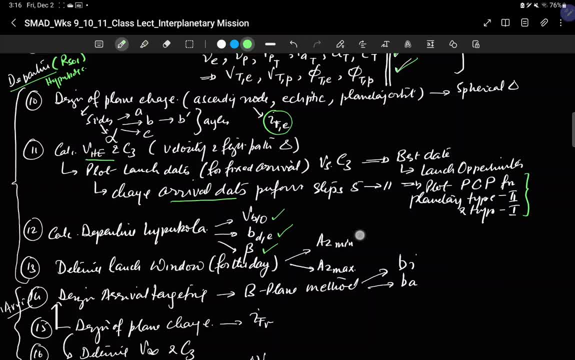 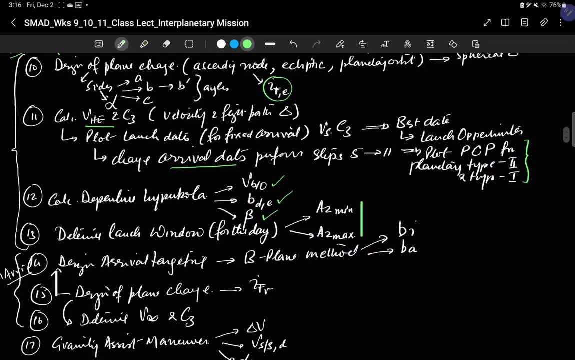 Has some thoughts And then, of course, saw we were able to also determine, as for the as much, the maximum, the minimum, as I, for the course required according to the rotation of the Launch port. now, today, what we will be doing is we are going to put together 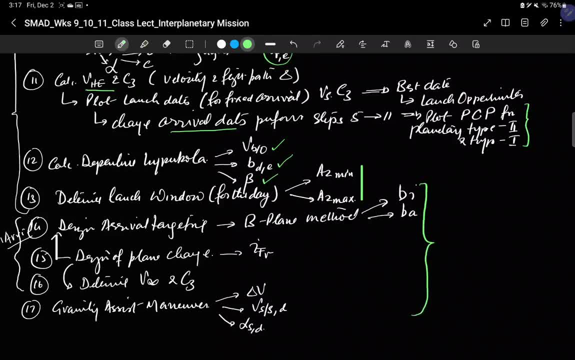 based on all that we have done, we will be doing the arrival trajectory calculation, and for that we will be using a B plane method, and then the rest of the calculations will follow the same method of the design of plane change, which will give us just like an ITE on the earth side. 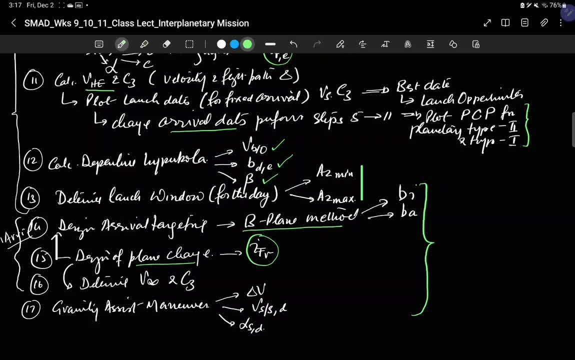 it will give us the ITV on the Venusian side. it will also give us the measurements, the magnitude of the V infinity, which is the velocity at the infinite location, and the C3, and after that we are going to do gravity assist maneuvers and make some variations. 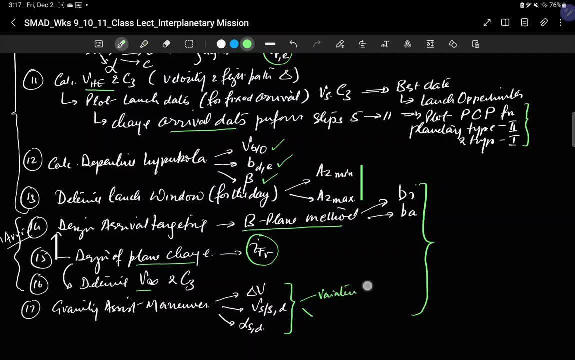 to this gravity assist maneuver in terms of the maximization of the velocity as well as the maximization of the turning of the spacecraft inside the gravity assist, because now this solution, so basically the step number 14 to 17 and onwards. this is all inside the 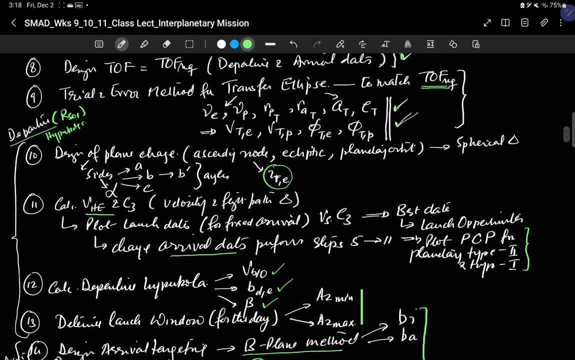 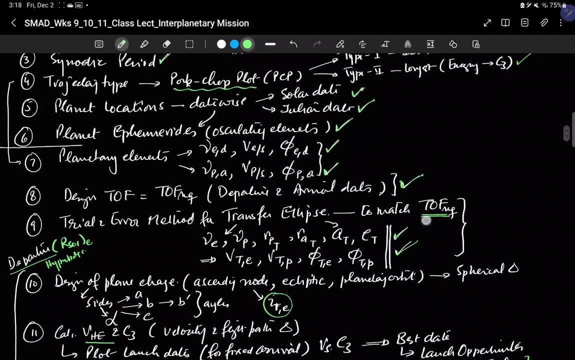 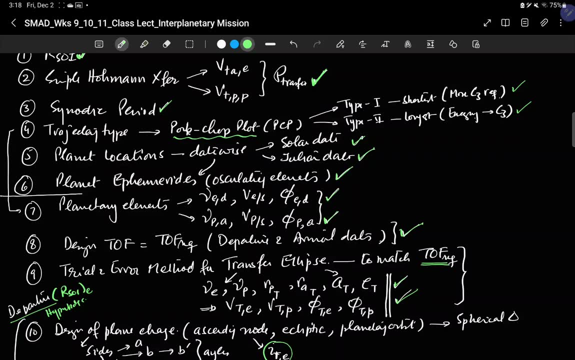 RSOI of the Venus, whereas the previous tests were all the departure tests were all inside the RSOI of the of earth and prior to that, all the calculations were done outside the RSOI of both the planets, but within the gravitational field of the sun. 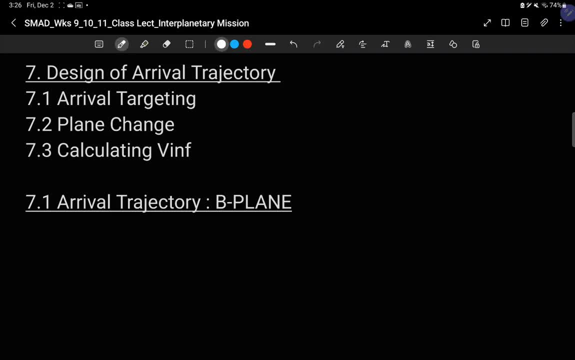 in the solar system. so let's start with the design of the arrival trajectory. now, this design of the arrival trajectory is done by a method. there are several methods to do this, but the one which is, as we say, very common is called as the B plane. and why do we do this? 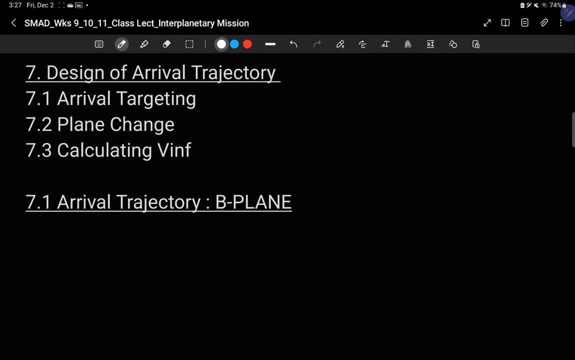 so the arrival trajectory. the reason we are doing the arrival trajectory is, first of all, we want to get to the target planet. but why do we wish to get to the target planet generally? one reason is that we want to create a direct impact. for example, you impact a. 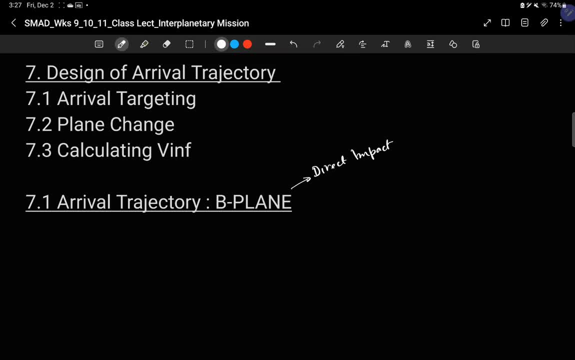 satellite onto the surface of a planet to see what is the composed of the surface itself and how does the impact occur. so there are many, there are many, many spacecraft that do that. they are which are bombarded. for example, the ranger spacecraft was bombarded onto the martian surface. then we had so many. other spacecraft and many of the rovers also do this after the at the end of their lives. so either you make a direct impact onto the planet or you want to use the planetary gravity cyst to move onwards for an interplanetary motion, so, for example, you get out of the earth's orbit. 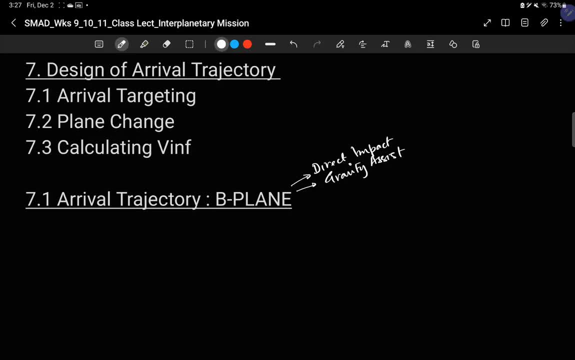 get into the venus orbit and it use a flyby of the venus and then you go on to another orbit and to another planet, and so on, so forth. you keep moving. for example, the voyagers mission uses spacecraft, different planetary bodies, to hop from one planetary body to the next planetary. so 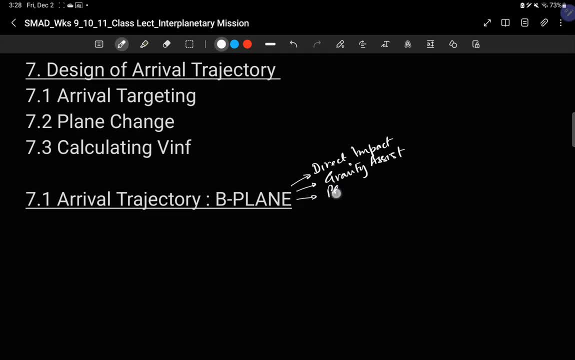 that is called as a gravity assist and the third is called as a planetary probe. so you enter a planetary orbit and you stay that in that orbit. and that could actually mean if there you have a probe, you can also have, you can also have some kind of a lander also which can just go on to the 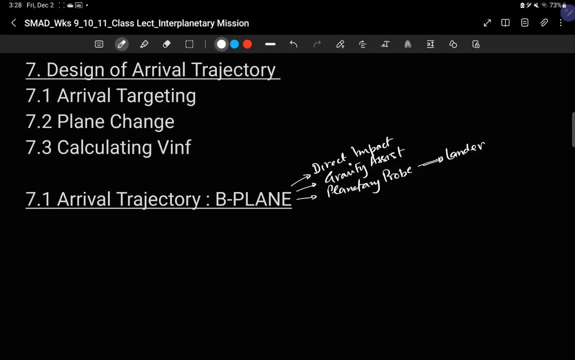 to land and using either the astronauts or some kind of rovers. so you, this lander, you can take the astronauts there, or you can take the rovers, and so and so forth, but the primary thing is that you have to bring the probe in. this probe is actually a remote sensing system, so it's a remote sensing satellite. which is now orbiting inside the, inside the orbit of that particular target planet, and so it's staying there. so there are three different reasons why we do that. and there's so many of these probes that we have- we even we have changafa four and five, which is the moon, uh, we have, uh, magnanion. 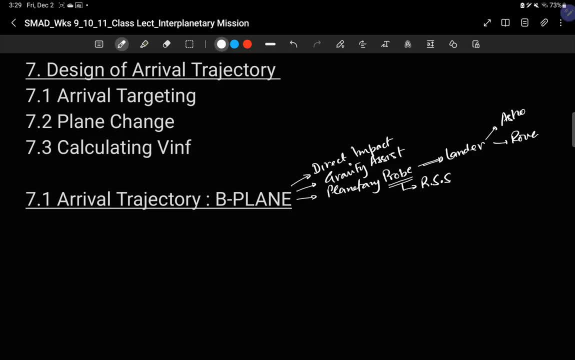 which is in mars. then we have the nasa probes that are in mars, and then we have juno, which was in uh jupiter's orbit, and so on and so forth. so the point is that we have to, uh, we have to do this by creating something called as an arrival targeting. 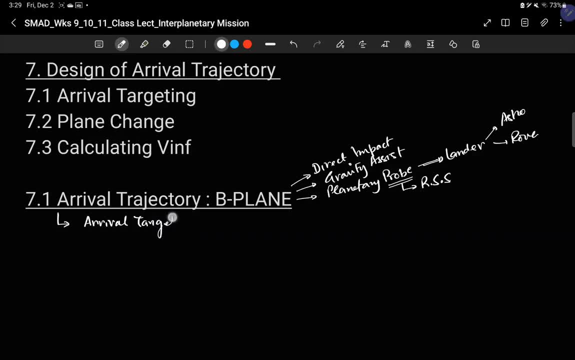 so arrival targeting means that you're going to target a particular planet, then you're going to arrive in a particular planet, and then you're going to arrive in that planet with the particular aim which is listed here. so these three things, these three types, primarily are your objectives, and so that will determine how you are going to, how you're. 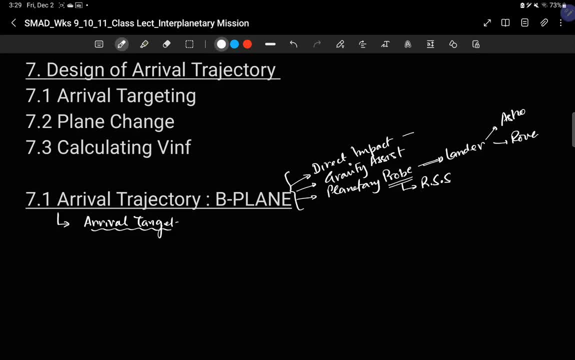 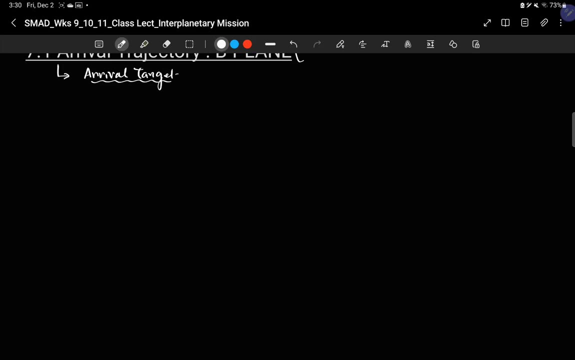 going to make an entry into the b plane. now, what exactly is a b plane? uh, basically, what happens is that you, we are placing an incoming asymptote in the desired location relative to the target plane, and so let's, let's do that. let's do that by drawing it, and we need to draw a couple of figures. 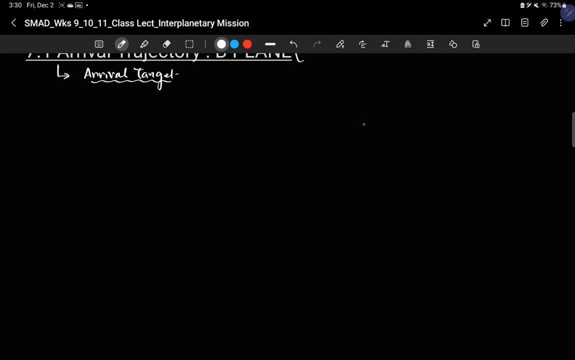 here, uh, so let's suppose this was our, uh, this was our target planet, okay, and it, the it's at a certain angle, which is usually, uh, true for almost all the planets. so they are, let's say, they have a certain orbital plane, and this orbital plane also contains the uh, the motion of the uh incoming spacecraft. 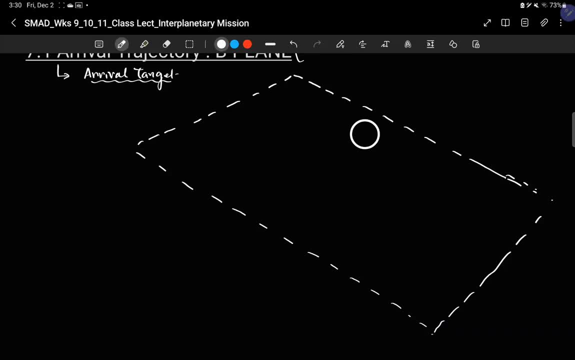 so we have this uh plane of this planet and uh, this plane also holds, because once the incoming spacecraft has arrived into the planet's orbit, so it is in the same plane as the target planet. so let's suppose this is our, this is our incoming spacecraft. it has arrived into the same plane, so there. 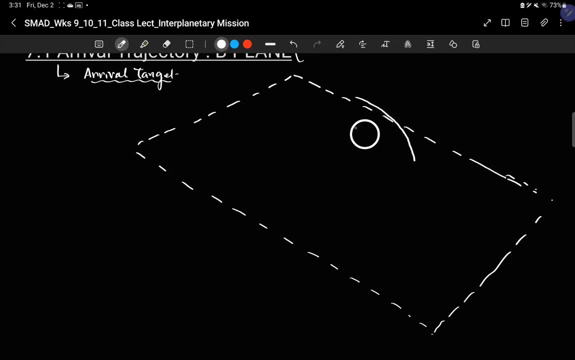 the, the host planet, as well as the spacecraft, and, uh, let's say this, uh, this is this whole, this plane is aligned with the equator of this, uh, of this uh target plane. now, what we do is in order to determine, in order to determine how this uh, what should be the distance? 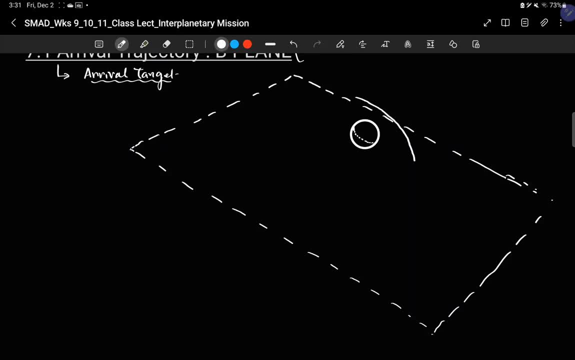 between the spacecraft and the host planet. depending on the three aims that we have set, we are going to make an uh, a orthogonal interception plane, which is called as the b plane. so we're going to make an orthogonal intercept plane here. so let's make. let's make it here. so 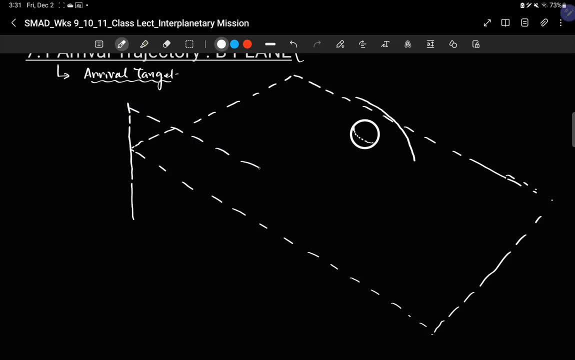 because this is at an angle. so let's say this is slightly at an angle and that's my intercept b plane. so i make a plane which is at 90 degrees to the orbital plane, uh, housing the spacecraft. so let's have these, let's mark these, uh plane. this is: 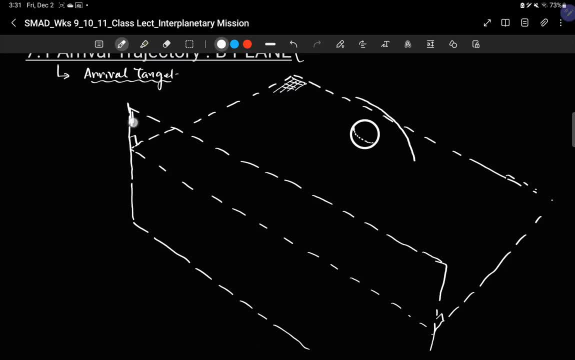 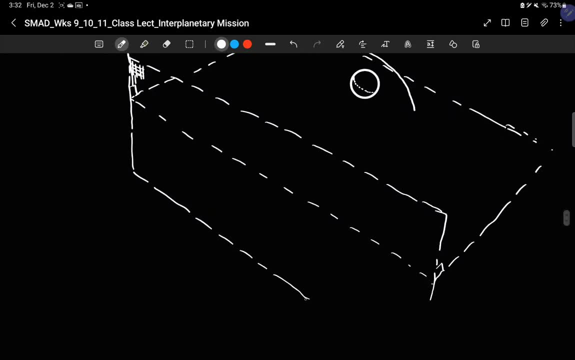 uh, this is the horizontal plane and this, uh, of course, would be our, a vertical plane here, so both are at 90 degrees to each other. okay, let's finish this. okay, so what happens is if i project the position of my satellite, of my host planet, here. so this is. 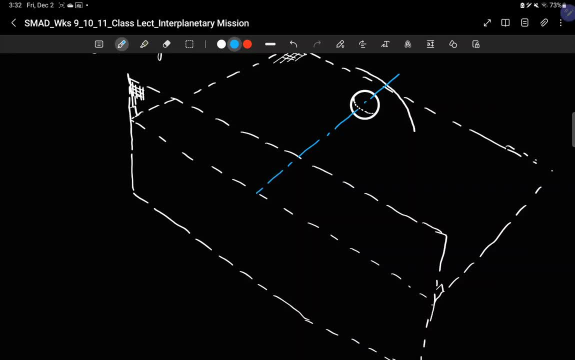 the direction of the propagated v infinity. why it is the direction of v infinity? it's because the v, the we have a v infinity of the satellite or the spacecraft which we are also passing through the same center of the motion of the uh of the central body. 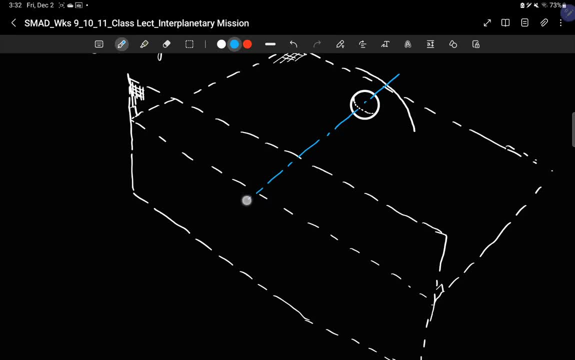 around which the spacecraft is moving. so this is the direction of the v infinity of the spacecraft and we pass it because we have to create a hyperbolic trajectory. for that, the v infinity has to pass through the center of the central body. this is the, this is the basic construct. 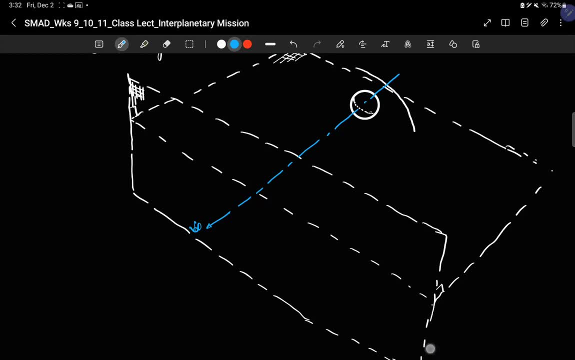 of a hyperbolic trajectory. so i'm passing this here and i can project the surface of this planet onto the b plane. so my b plane is orthogonal, so i. what happens is that this same surface is now shifted 90 degrees. so i'm gonna have to make a superconductor. so what i'm gonna do is i'm gonna 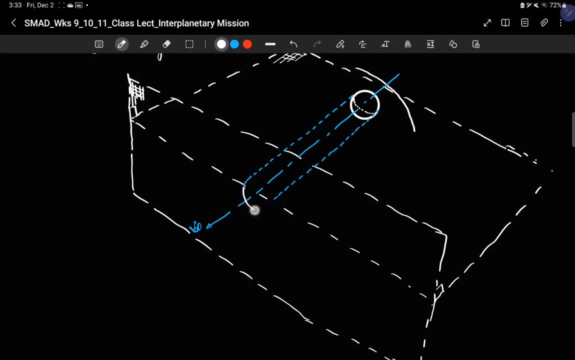 So I have, I will see this surface here in 90 degrees in this manner. So that's my, that's my surface. So let's just highlight this, Okay, and this has an orbital radius, let's say r naught, which is projected onto the plane. 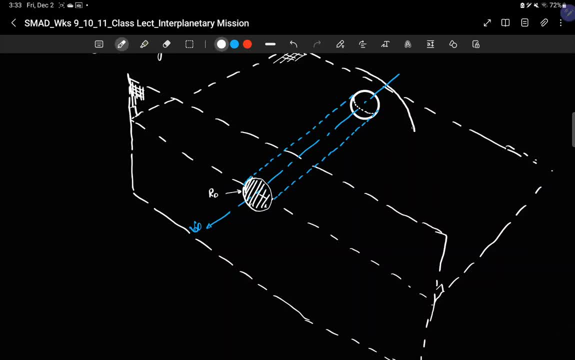 and now let's bring the spacecraft in. So the spacecraft comes in, and along the hyperbolic trajectory, and so at this point it becomes parallel to the V infinity. So this is the V infinity, and this is this. has you know, it crosses the B plane. at this, 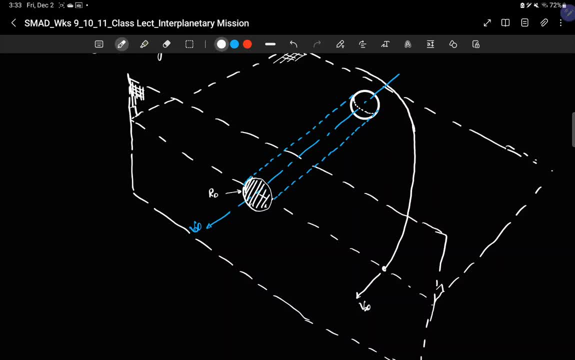 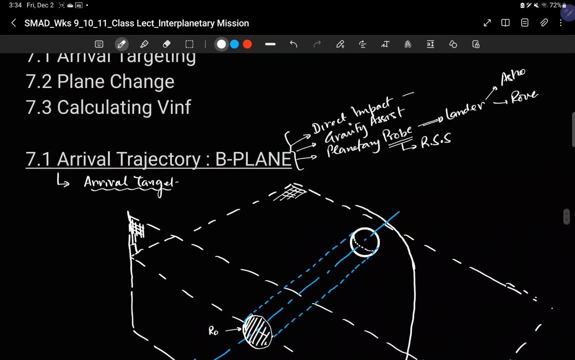 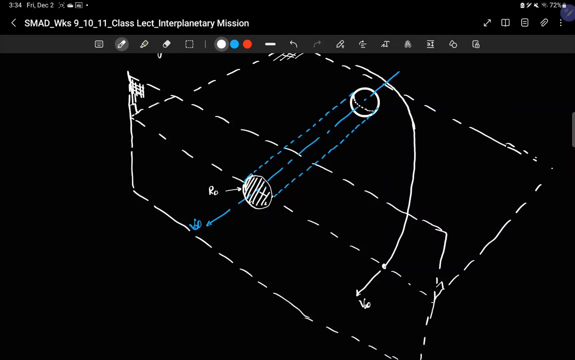 location We can call, give it a number or something, but this is the position of the crossing of this B plane. Now, in order to determine whether it's an impact spacecraft or a gravity assist will determine How much is the distance between the spacecraft and the surface of the planetary body. 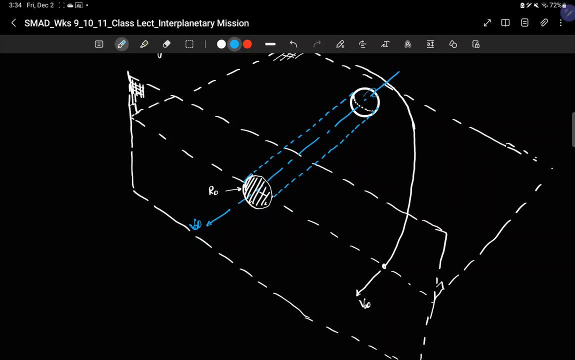 So let's, let's project now the path of the planetary body. Let's say, this is our path of the planetary body and I'm projecting it here also onto the B plane. So this is where the center of the body goes. So the surface of this, of this planetary body, will intercept this B plane at this position. 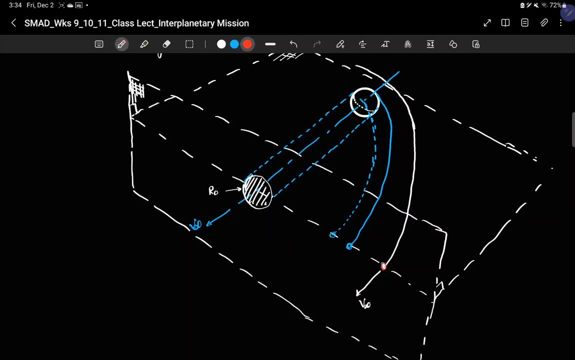 So now we have, We have two distances: We have the intercept of the, the intercept of the spacecraft following the white trajectory, and we have the intercept of the planetary surface, which is in the blue, So the planetary, so this is the surface of the planet. 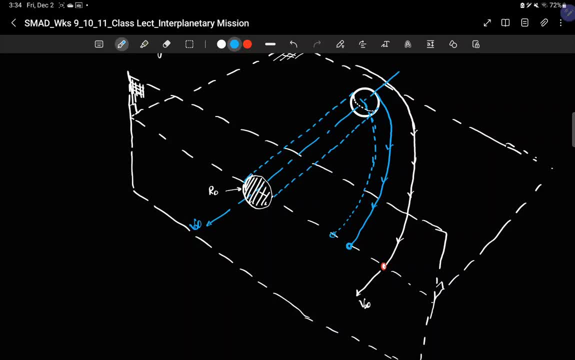 So there is a difference between these. the difference the distance between these two is is very, very significant and important to us. Now, you know G, please, Sir, This planetary Intersection point that we have taken. It means that if the planet were to follow the same trajectory as the, 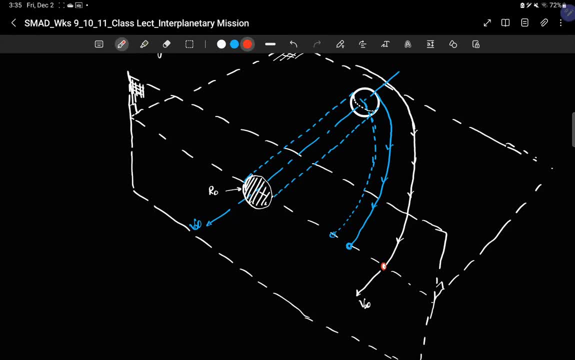 No, no, The planet is already following its own trajectory, So it's possible. This is where the planet will intercept this B plane. Okay, Because we have to calculate the distance that is required to either impact, use a gravity assist or get into a planetary probe. 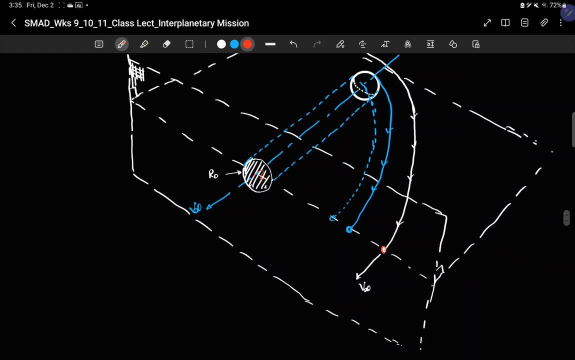 Okay, So the distance is very significant for us. So to do that, Let's now put some coordinate systems here. We usually put a coordinate system which is called as R and T coordinate system. R and tangential. So this is R and T coordinate system. 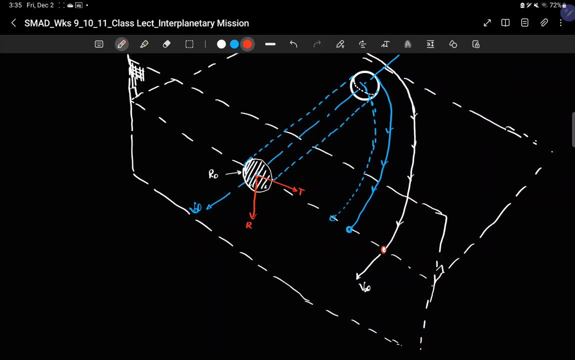 And this coordinate system will help us determine the magnitude of the distance between the two. So this distance between two V infinities. So I just let me just project this outward. So the V infinity here by the basic geometry of the hyperbola is called: this is the semi. 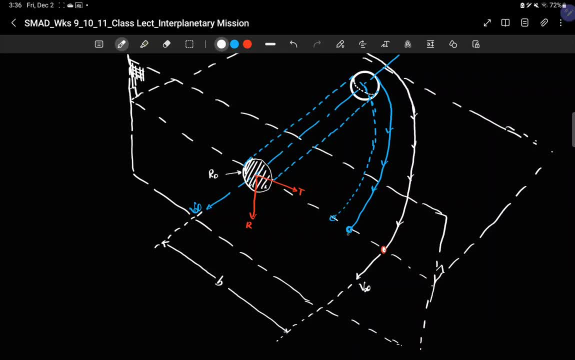 minor axis. That's the basic geometry. So by that extension, by the same extension, the surface, this is called as the semi major axis of the impact. So we call it BI. So that's the semi major axis of the impact, exactly the surface. 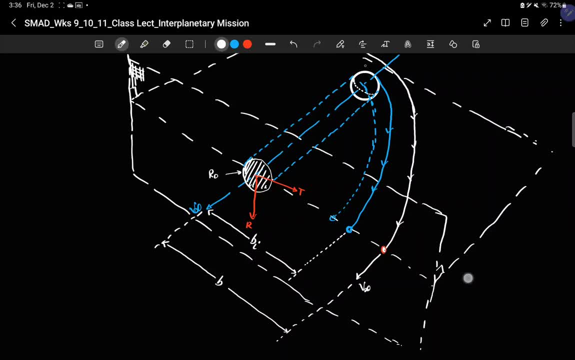 Now very close in magnitude to this is, let's say, there's an atmosphere. if you are looking for a probe, So then you should also be interested about what is the, What is the atmospheric height around this, around this planet? right, In that case, the same BI will have a corresponding value, very close to it, but greater than that. 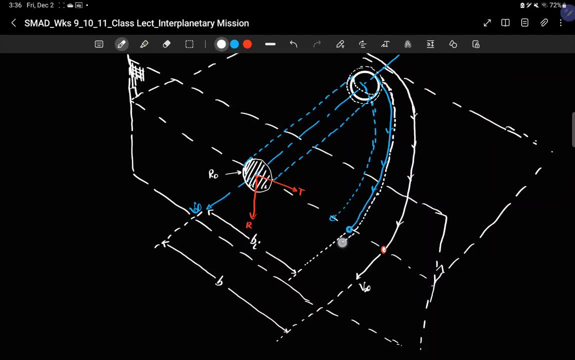 will be another semi major axis and that is called as the semi major axis of the atmosphere of the planet. So it's called represented by BA. So we have a B, which is the semi-minus, Semi-minus axis of the incoming spacecraft. We have BI, which is the semi minor axis of the exact surface of the planet, and a BA. 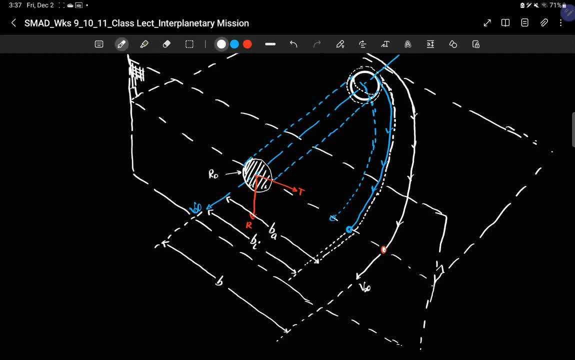 which is the semi minor axis corresponding to the atmospheric height. So we can So the idea of a B plane by solving this B plane actually, so, which is of course the- we have seen that this is a. so by solving this plane, this whole orbit in a B plane, makes the orbit becomes two-dimensional and white becomes. 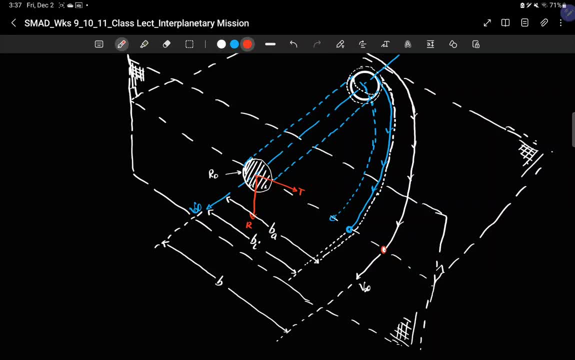 two-dimensional. So if I was checking this planet, for example the motion of this planet on the surface of the B plane, then it would appear to be as two vertical lines. For example, the planetary spacecraft will appear to be on a two-dimensional plane as this and that. 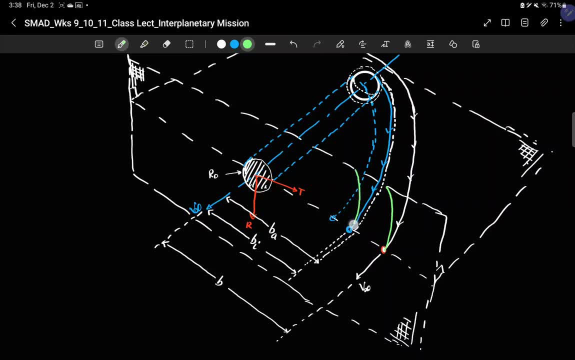 of the planet will appear to be another one like this. So when you map, because this is coming in, but this is only possible when you are mapping from a very large distance, mapping from a very large distance, So, and any variation in the incoming plane, any variation in the incoming plane, will be accounted for. 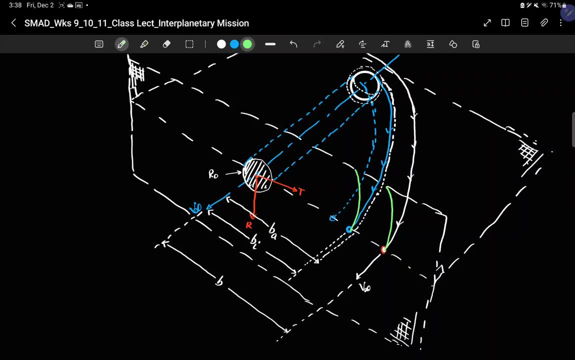 on this on the surface. So you may not necessarily mean that will mean that you may not necessarily have these two planes at 90 degrees in that case, because only then you will be able to map these two surfaces. because it may be coming in at a certain angle and this is what 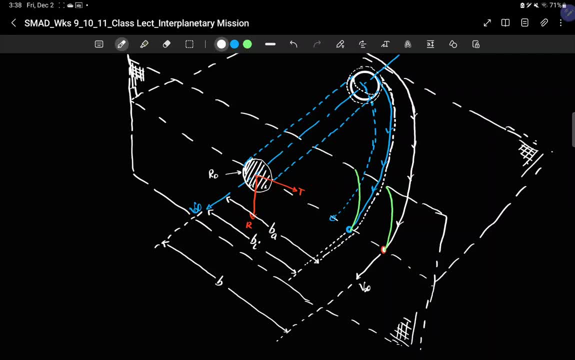 is happening? This is what is happening because this plane, this plane, the B plane, is orthogonal to an infinite position. So this is primarily orthogonal to an infinite location, but your incoming, but your incoming plane is at an angle. Why? Why was it at an angle? Because 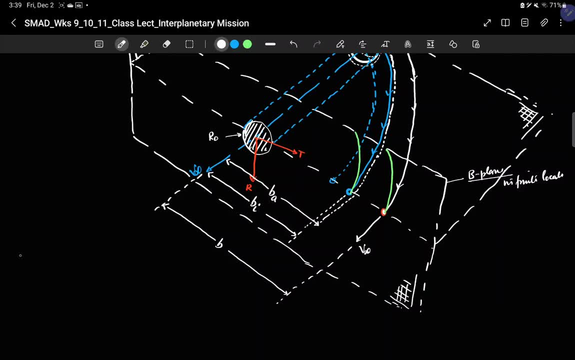 if you remember, when we, when we calculated the orbit, let us say that was the earth and this was Venus, and we had the two orbits, which were in two different directions. So the earth had a orbit in this direction. this was the ecliptic of the earth, and then there, 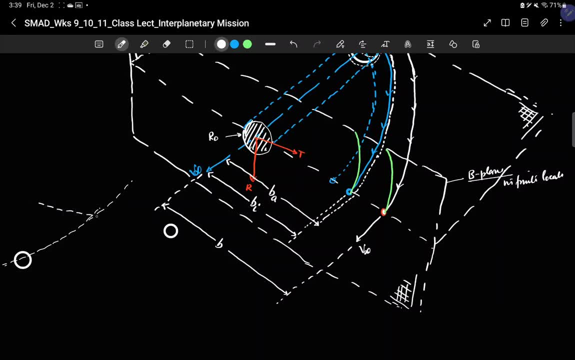 was an orbit of Venus which was at a certain angle to the ecliptic. It was at an angle to the ecliptic and so we joined that. card leaves here will follow a trajectory all the way and we calculated this triangle. 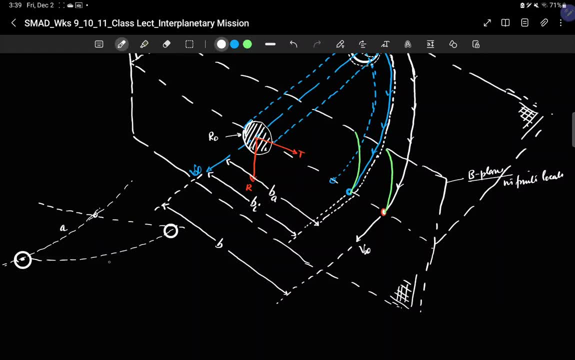 this spherical triangle where we call this as A, we call this as C, we call this as B, if you remember, and this was the angle alpha and this was IT at the earth side and this was IT at the venusian side, which means that on the venusian side, when you draw the B plane, 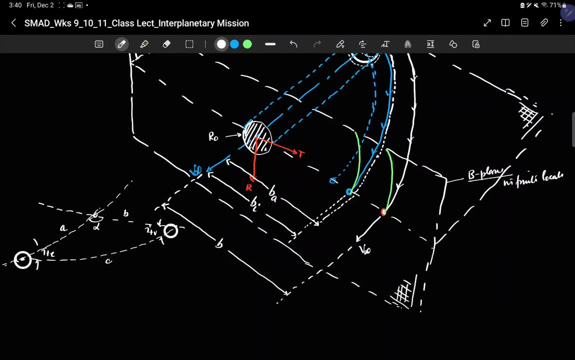 this incoming plane will not be orthogonal to it, because this incoming plane will now be at an angle ITV till the spacecraft has exactly reached the surface of the plane. only at that point it will be in the same plane. So the spacecraft is actually coming down and trying to meet. it is coming down, let's. 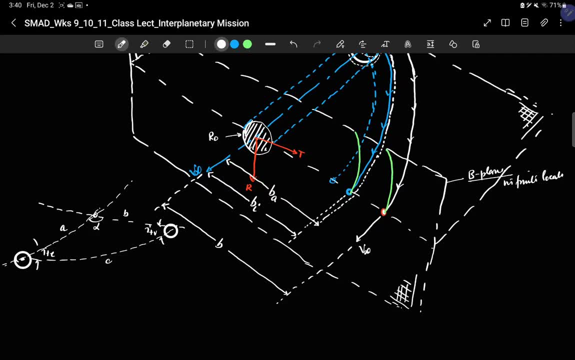 say, at an angle and trying to meet the orbit plane of the target planet at point B, and if you project it And then it will cross underneath this planet. so this is the basic concept, so that why, when we look at from the same B plane, we will see that the entire trajectory of the planet and 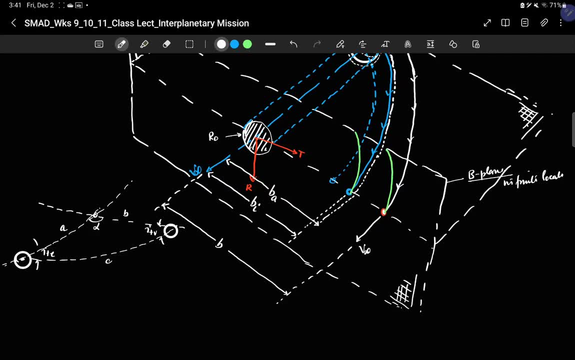 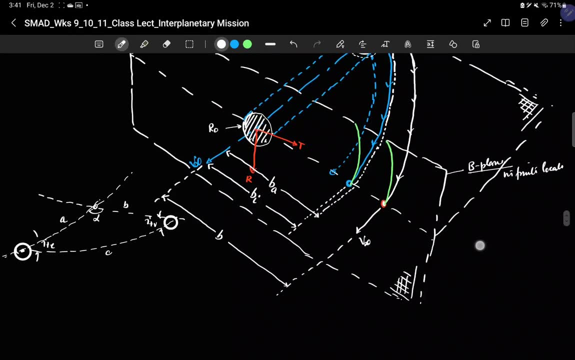 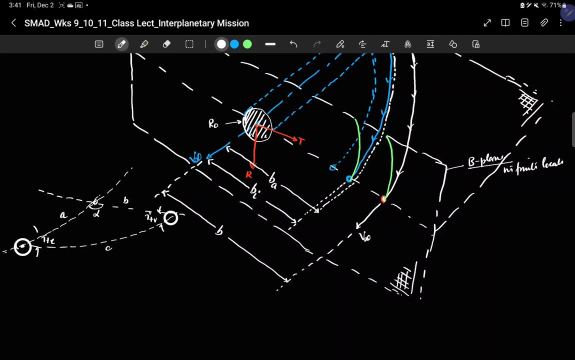 that of the spacecraft, can be met by these two lines: onto the plane, onto the B plane. So the B plane now houses the trajectory in two green colors: the trajectory of the planet and the spacecraft. it houses the position of the satellite, The target planet and the intercept positions of the spacecraft and the surface of the planet. 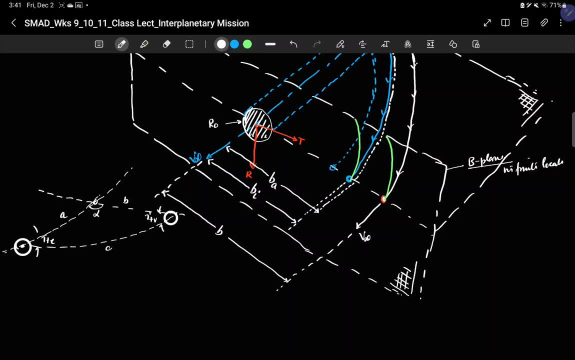 yes, please, Sir, correct me if I am wrong. if we were to take this B plane exactly orthogonal to the planetary curve, let's say, then you will not see this point, then you will just see two points, two points. you will not see any line. you will see actually. yes, in that sense you 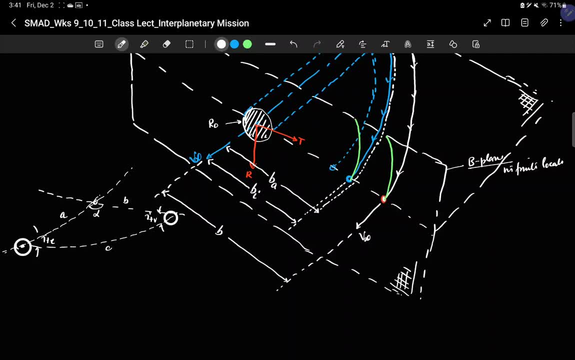 will see a line, exactly an elliptical line, So the inclination that is constantly changing as well. so this B plane can be said to be taken onto the spacecraft. can we say that we are looking from the spacecraft towards that planet? Now you are looking from an infinite position onto this spacecraft arriving onto the planet. 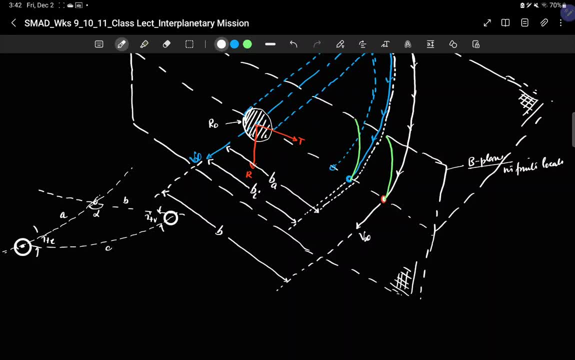 you are standing infinitely far from that place And looking at the arrival of the spacecraft into that plane. and now, because that distance infinite, you are looking at a position from where the two planes will cross, where the two trajectories will cross, So you create a plane there. if that plane is, if that plane is orthogonal, then it will. 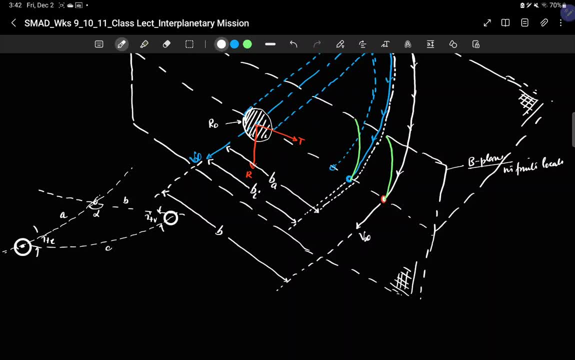 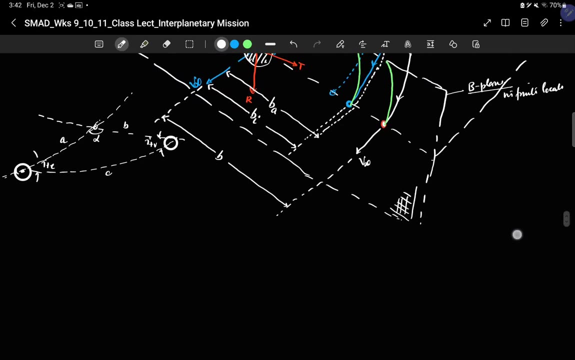 create a ellipse type on effect. if it, if it has non orthogonal and it is orthogonal only to an infinite location, then it will create lines, these kind of lines here. So it depends on how you are placing that orbit, that plane. the objective here is that we need to calculate the B value, the BI and the BA. so we have three things to calculate. 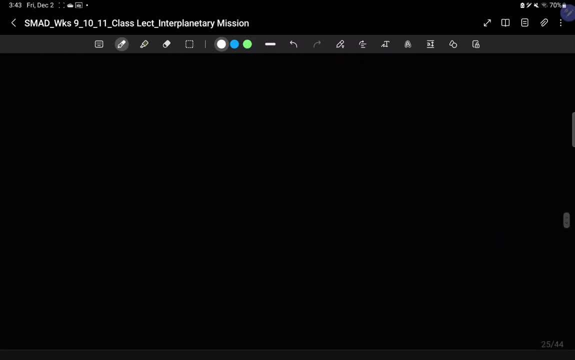 here and, as I mentioned that, if we were to let this thing project, then how will it look from this position? let us say I am, I am on the B plane, so this is what I am going to calculate. Okay, let's just look at the three-way positions. 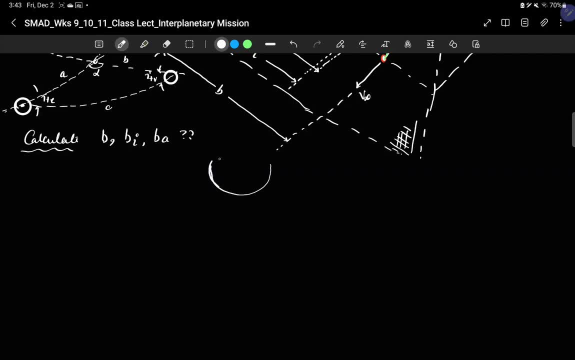 For example, this is Venus. This is Venus mapped onto the B plane. So when we have Venus mapped onto the B plane- so I put this Venus, I'm just putting the half of it- then the incoming spacecraft is at a distance, let's say B, from here. 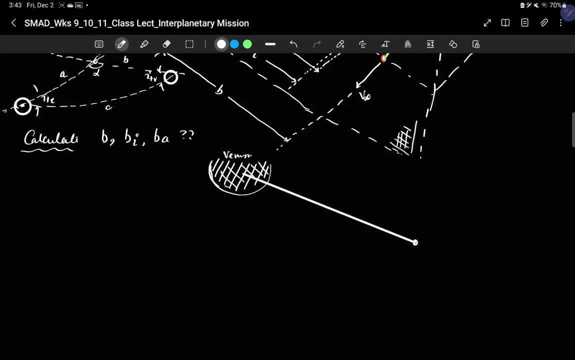 That's the position of the spacecraft And in order to get to this position, the spacecraft will be going through several adjustments, And we call it the course corrections. So those corrections will appear as, as we mentioned, will appear as a set of concentric ellipses. 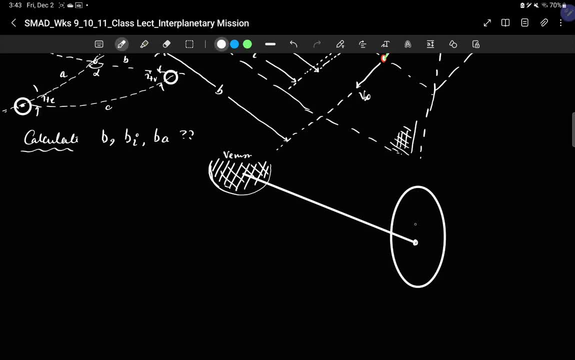 So this may be the first ellipse, the first correction. Then, in order to cross this, there will be another correction, another ellipse will be found And finally we reach the corrected position. So if you were to draw this, then you will find that there, the R. 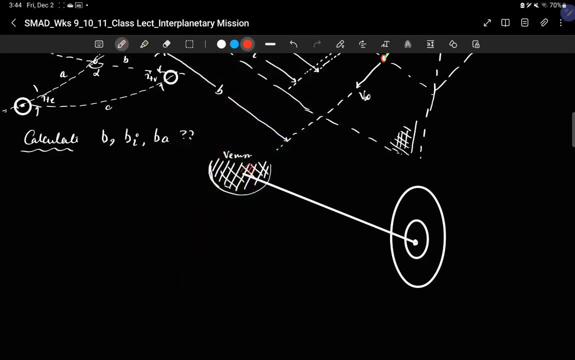 that the R coordinate system, that was R- will be pointing in this direction, And we have the T which will be pointing in this direction. So in this way you can have the incoming spacecraft. So this is your B here. Okay, 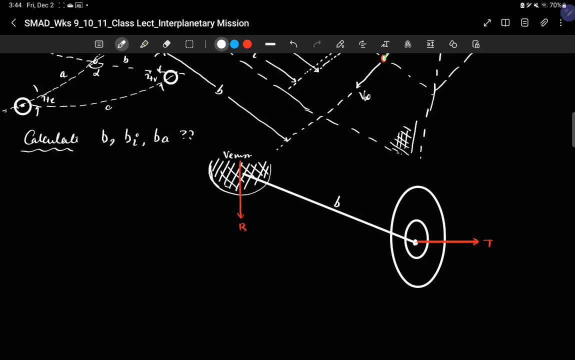 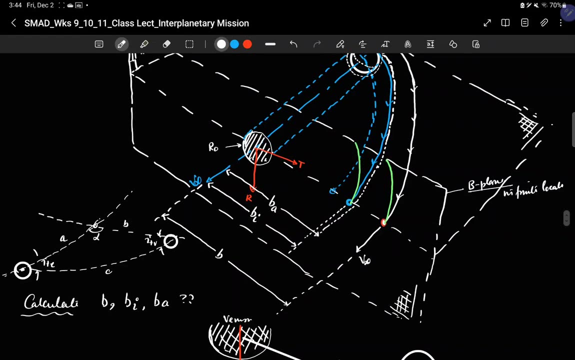 So this spacecraft can be at any position above or below that. So because, remember that this depends on the inclination of the host planet. This depends on the inclination of the host planet. Okay, So that is why, even if you put this orthogonal, even if you were to put this orthogonal, 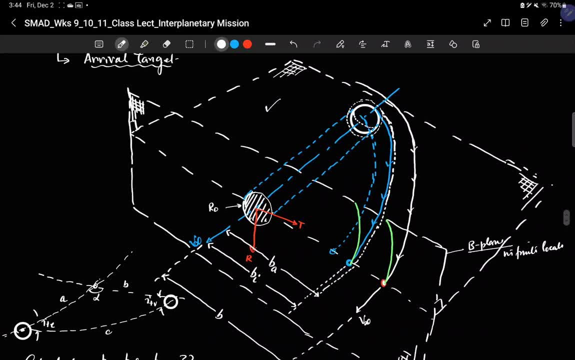 because the host, because this plane is angular to the orthogonal to the ecliptic. This is orthogonal to this plane, which is at angle, And it is also. it is in line in the same plane, its equator is in the same plane. 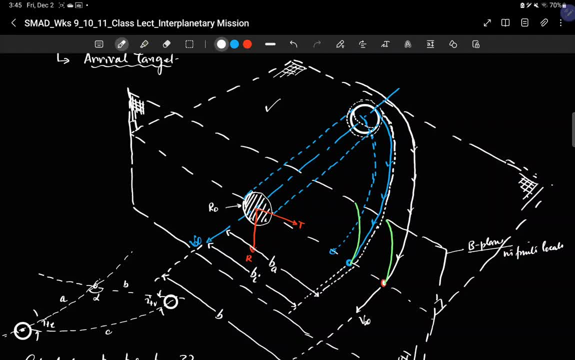 and it is in the same plane. So this is the same plane, And as the ecliptic. So therefore, these lines will invariably appear on this thing, because your incoming plane is at an angle. So this is how the lines will appear to exist on this plane. 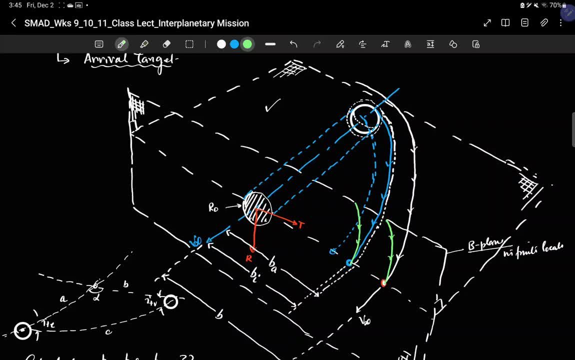 because now try to imagine that you have a plane and the incoming plane. it is an angle and the intercept is at 90 degrees. The intercept is at 90 degrees, So any trajectory map there will still, it will still be mapped as a line onto this plane. 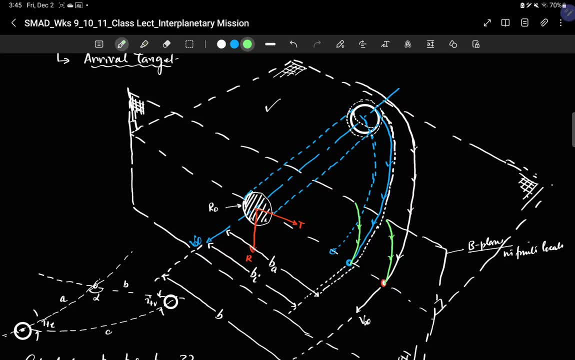 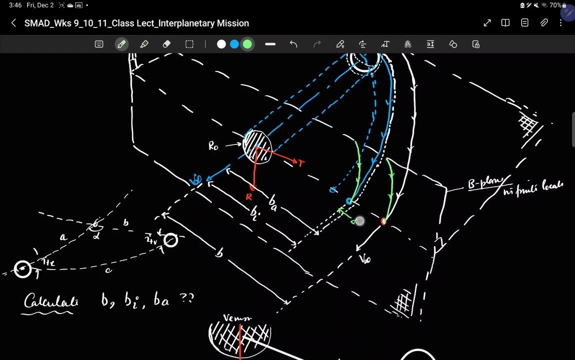 So these lines will appear in any generic case where you have a, where you have a inclined plane attached to the B plane. So the idea is that if we have, if we have to adjust this distance between the two planes, let us call it the delta B. 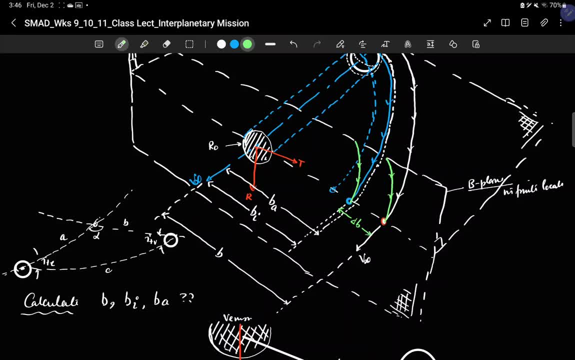 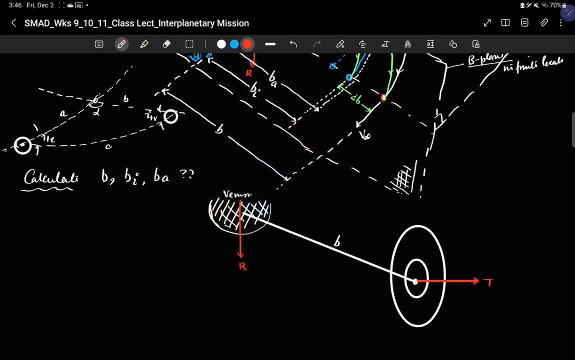 So this delta B will determine what kind of a mission we will be performing, And that is why your R, your R vector and the T vector. So the T vector was in this direction, So you can have your incoming spacecraft above and below the planet. 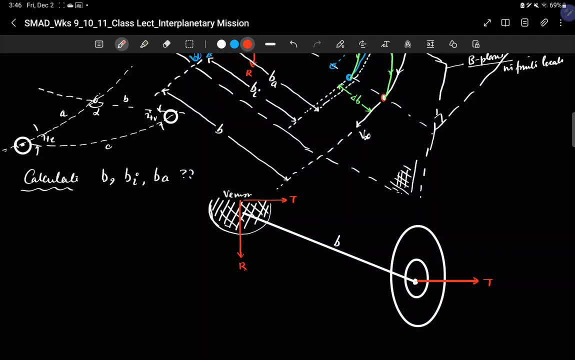 because it is coming down and then it can go down and then it will create that. it will create the orbit around this thing, which can be an inclined orbit. So if it is an inclined orbit, so then this will go around this space. this orbit, and the R and the T which are on the B plane will be at an angle to the space. 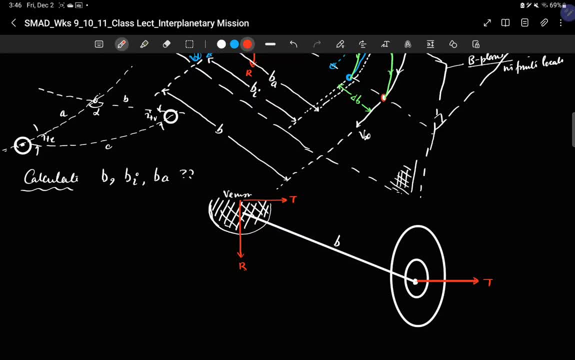 spacecrafts orbit. okay, Sir, if we are having on that V plane- we are seeing those, the trajectory end points as one point, the end point which is actually on the V plane- then why are we depicting them with these ellipses, sir? Why not similar In order to get to this? 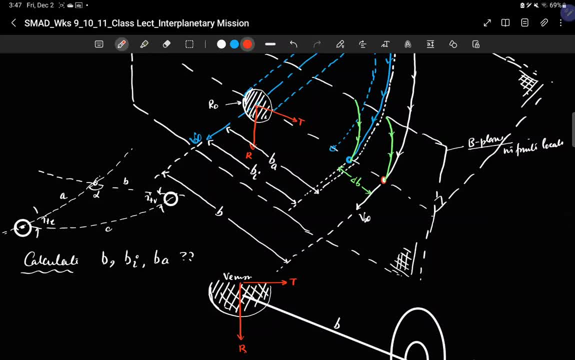 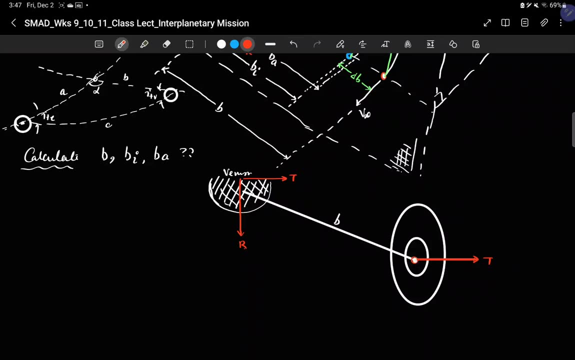 point. in order to get to this point, a number of course corrections are introduced. So those corrections, they create a kind of an elliptical motion. So what we are interested in is getting to this point, which was actually on this B plane. 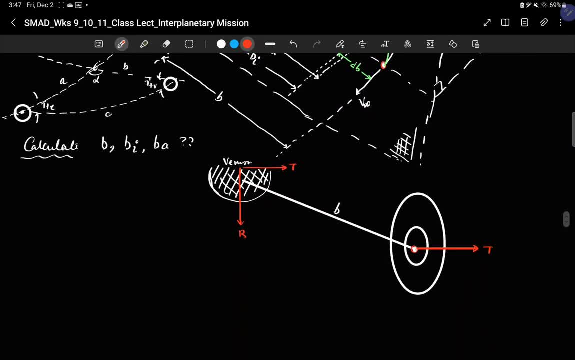 Sir, we are just trying to have, we have the same inclination as the planet's orbit. Is that right? Yes, When we are drawing this ellipse: Okay, So they are A and T, they are in the B plane. Okay, They are in the orthogonal plane. But the orbit? 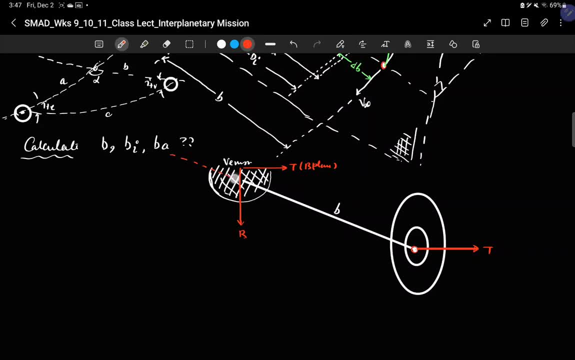 of the space of the planet can be is possibly this one. This is its plane. So the spacecraft is in the plane of the orbit, is in the plane of the of the planet, But the B plane is orthogonal to this plane. Okay, 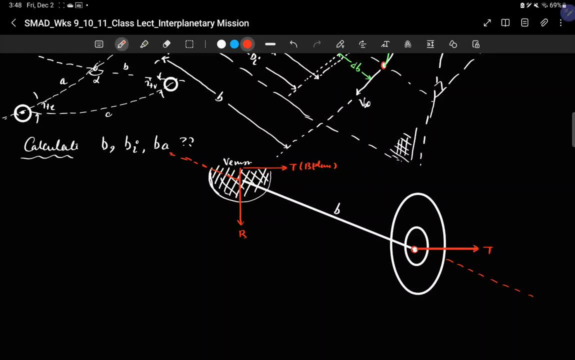 And these ellipses, the ones you have drawn at this point, the T. These are called as course corrections. Okay, In order to make sure that you maintain a B and a delta B is maintained, you have to make the corrections to your course. So every course correction will appear to be a set. 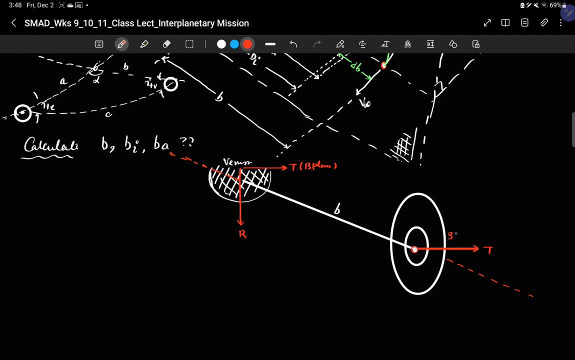 of ellipses with we call it three sigma, three sigma corrections. So we introduce the three sigma corrections, which is standard deviation in the correction data till you actually home onto that exact point. What is the reason why we need this? 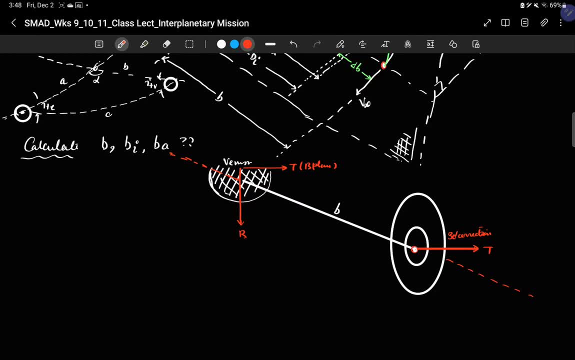 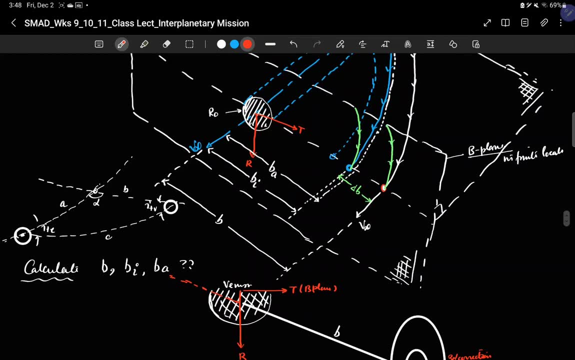 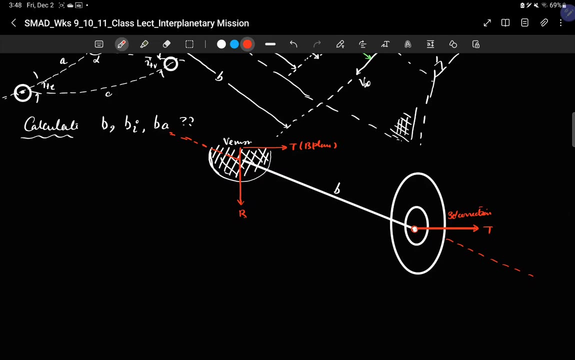 Because you're coming from a very long distance, So you have to make course corrections in between to make sure that you get to the right point. Okay, So, orbit: the insertion to the orbit has to be very correct. Okay, Now, in order to: in order to calculate this thing in addition. 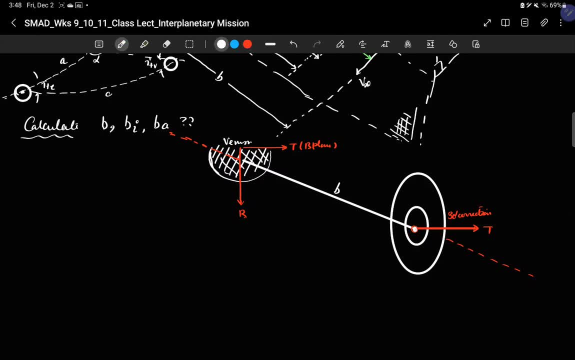 to whatever we have already mentioned, we will. the first thing we do is as a matter of process, once we have the B plane established. So after the bleep in we will do the plane, the plane change calculations, And we have already learned what we do in the plane in. 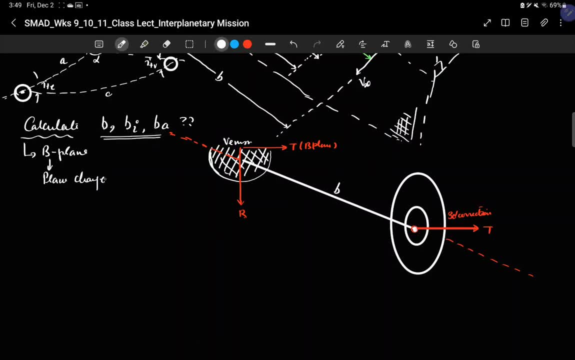 order to calculate these values, these variables, we must first do the plane change calculations. And those plane change calculations will give us the ITV, will give us the alpha at the arrival, alpha at the arrival, And it will also give us the V infinity of the spacecraft. 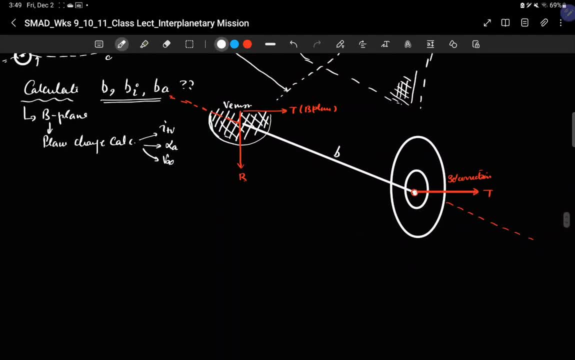 on its arrival into the planetary body. Okay, So, if you can always use the hand, the hand, the handouts for the for the hyperbolic orbit. So in order to get the value of B, any B is actually determined directly from any relations which has RP into for a hyperbolic orbit. 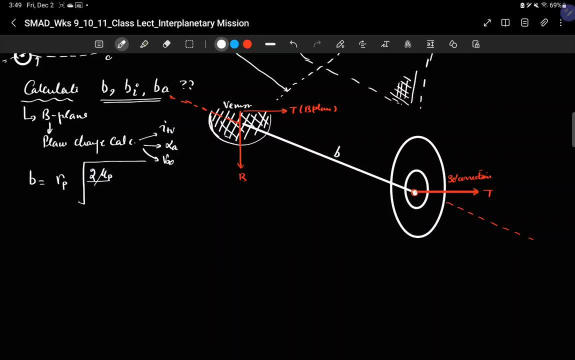 RP into 2 mu of the planet, 2 mu of the planet, whatever planet it is. RP into VHE square plus 1.. That's your relation for the hyperbolic orbit. We already derived this. Now in order to do, for example, the BI calculation: what will happen For BI? some corrections: 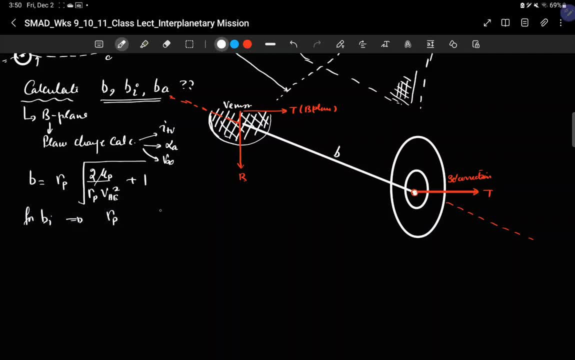 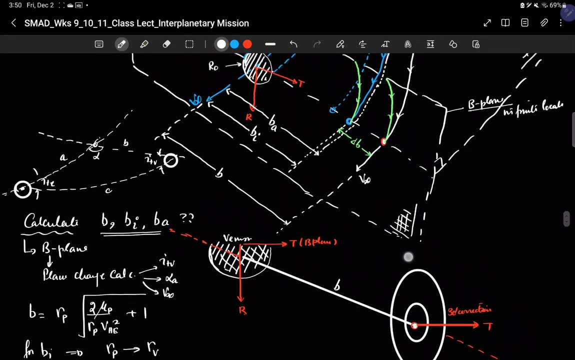 will be made. For example, we will change the RP to the. we will change this RP for the radius of Venus. We will change this to the radius of Venus because then the periapsis, because then we will assume that it's going to impact onto the surface and therefore we 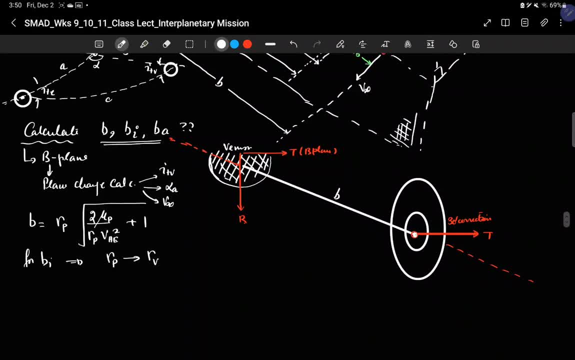 will use the RV value. The mu will be used as it is, The VHE instead of VHE. this is at the departure. We will replace this at the arrival. We have V- infinity at the arrival, So we will replace the VHE. 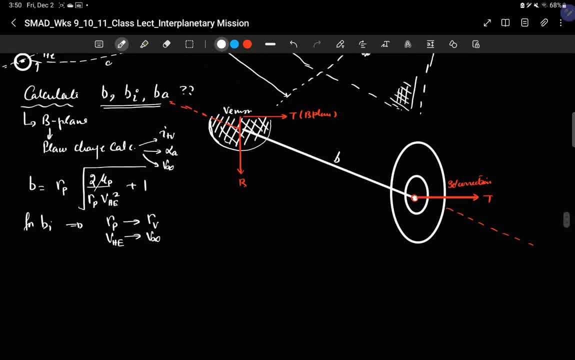 with V infinity. So that means, since we have, we can calculate the value of RV. that's not a problem. The value of the RV is about 6,052, the RV- sorry, this RV, capital RV- is 6,052.. 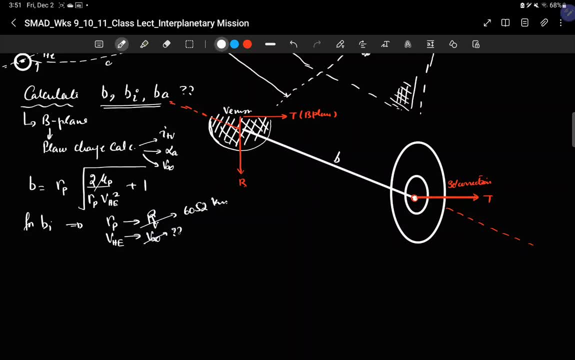 So we have 6,052 kilometers for Venus, But what we don't know is what is the value of V infinity here? Just for record purpose, the mu of the planet is that of mu of the Venus and which is very close to that of the Earth: 32485, 8.8 kilometer cube per second. 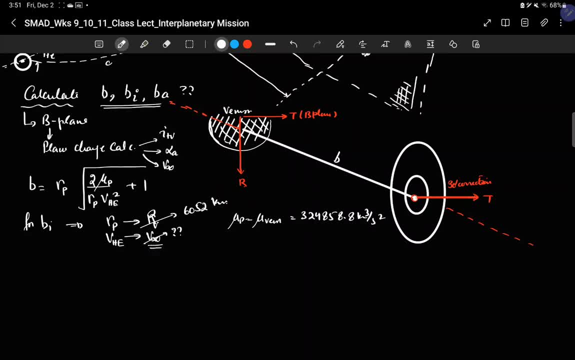 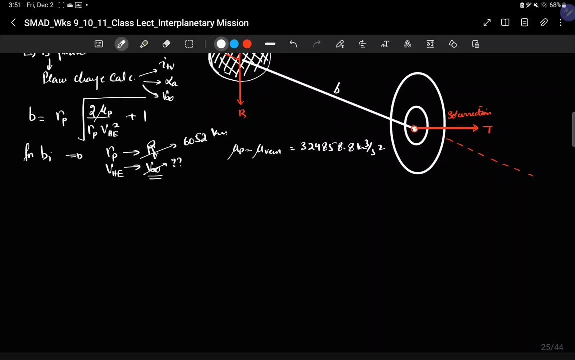 square. So, therefore, now we have to find the value of V infinity. This V infinity depends on our arrival at the planet. Okay, Okay, Yes, and we'll do the same triangle calculation that we did the last time. So we already knew. 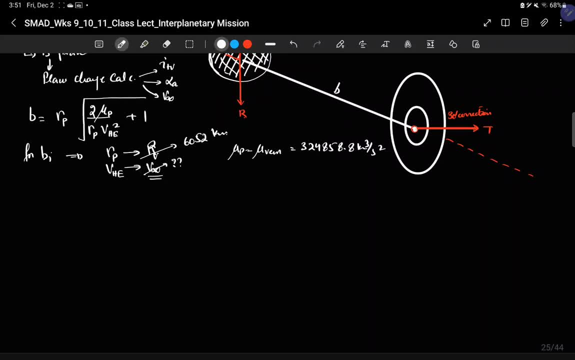 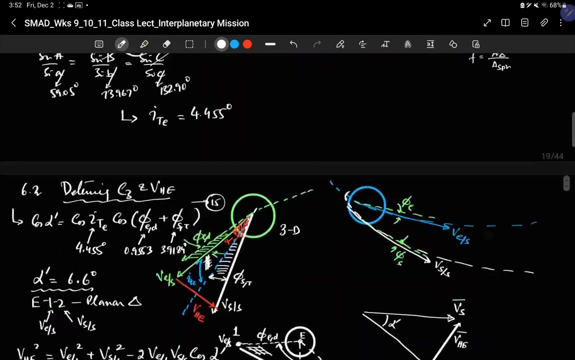 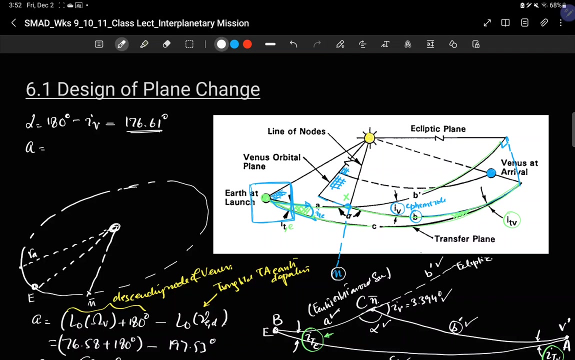 what the? so, in order to calculate the value of V infinity, we first need to establish the magnitude of ITV. So let's do that step first Now. so if you remember, I just recall the old figure here, Yes, this one. So I'm going to just draw this triangle which we used for last time. 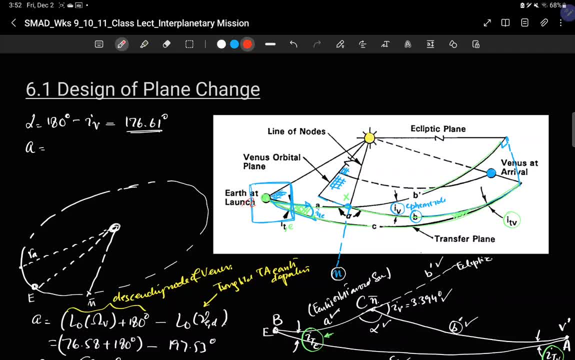 the calculating from the Earth, launch from the Earth end. That was one corner. The other was the projected corner of Venus. And then there was a node, ascending node, where the ecliptic was crossed by the by the Venus orbit projected Venus orbit. So this triangle, 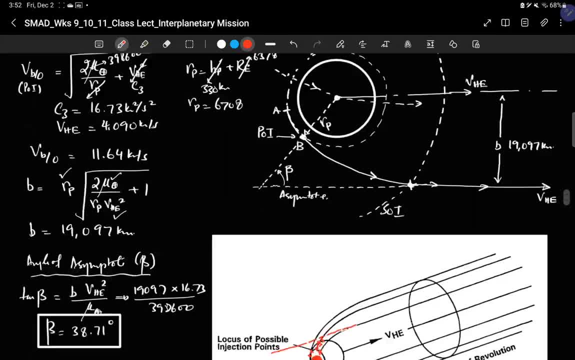 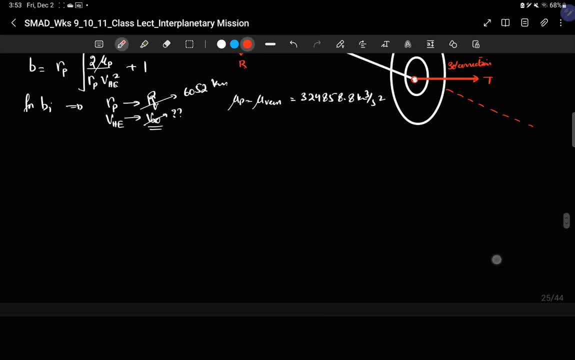 was solved last time. So we're going to use the same triangle, because it has departure inclination at one end and arrival inclination at the other end, So we can very conveniently use that. So on the arrival end, what will happen is we will have. we have, for example, this spacecraft. 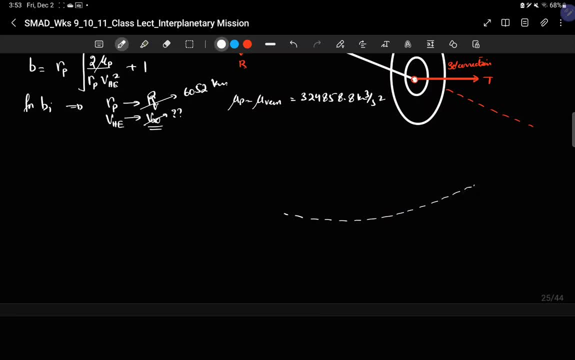 coming in and and we also have the planetary orbit, So the planetary orbit was in this corner. So this was the rightmost corner, the arrival corner isn't it. This is the center of the planet, for example. So this on the, on the, this was the arrival velocity. 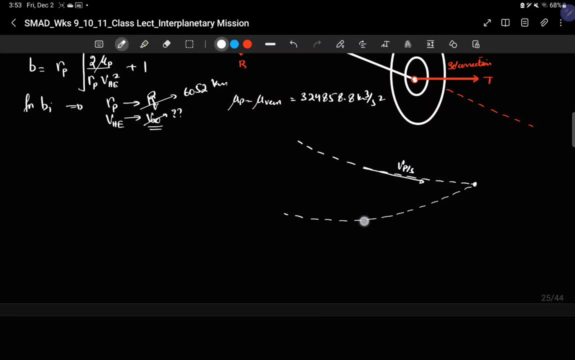 of the planet with respect to sun And on this side was the arrival velocity of the spacecraft with respect to sun. at the arrival point And the angle that we had calculated between these two was I on the transfer orbit, ITV, So it was the transfer orbit. 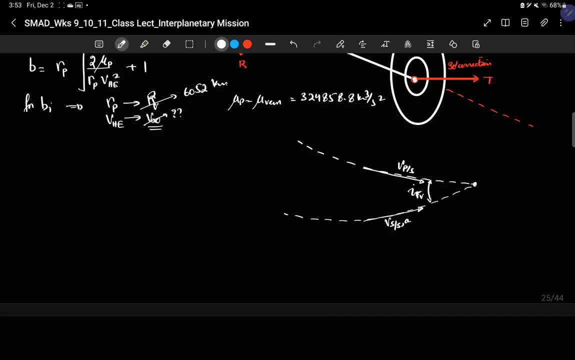 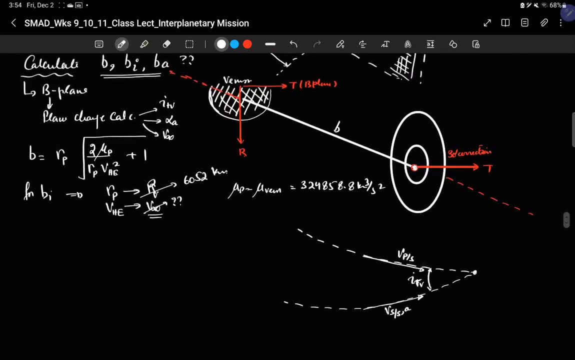 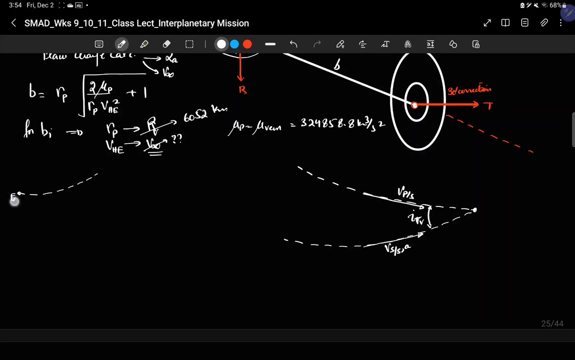 the inclination ITV. Now, just just if you want to remind recall, we had this figure. okay, This is this. this big figure is part of the same triangle that we had used. This was the Earth. here There was an intercept N, or we called it the point X, And then this: 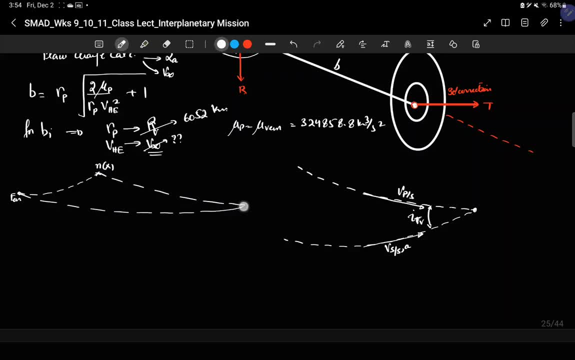 this was the intercept with the venous side. so this was the trajectory of the traversing trajectory. this was venous on this end and this end was ITV. we had A and B and C and we had an alpha here and there we had an IT of the earth. so what we have done is we are. 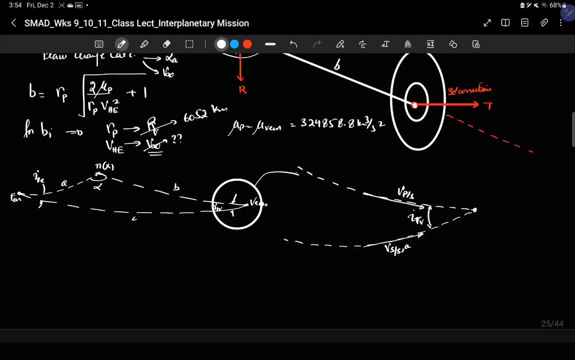 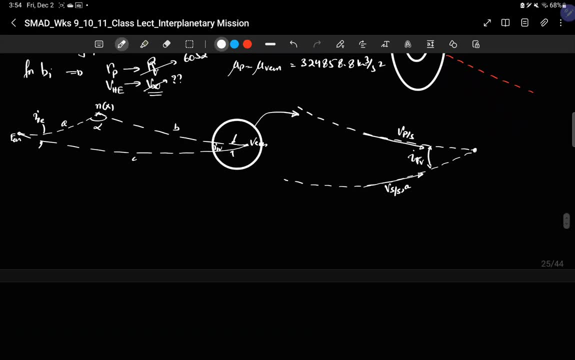 just solving for this corner and this is the figure representing this small corner. Now, when we solve for this corner, at that time we could use the sine rule. the spherical sine rule could be used, for example, on this triangle. we can use that. we have sine of. 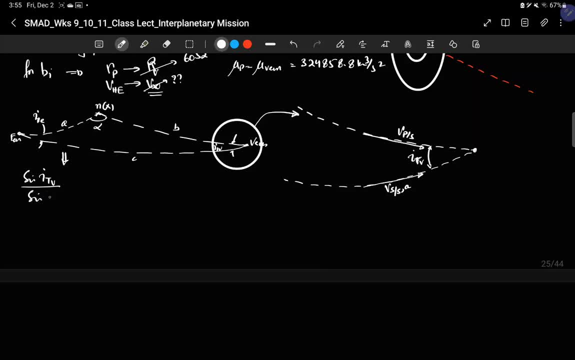 ITV over the sine of A would be equal to sine of alpha over sine of C. and if you remember from those last previous calculation, the value of A we had found to be 59.05 degrees, we had determined the value, The value of C, to be 132.90, please check your previous calculations- and we had determined: 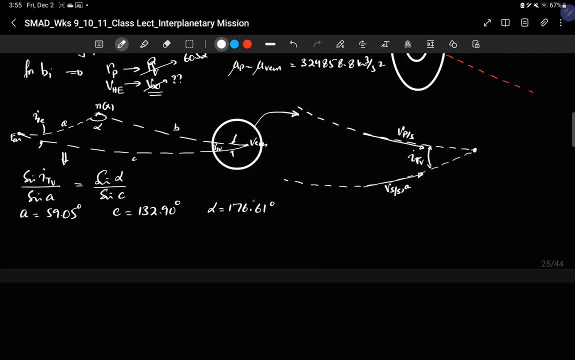 the value of alpha as 176.61 degrees. so therefore the unknown ITV can be determined here. so you will get the value of ITV as sine arc sine, which will be sine of A, sine of alpha over sine of C, and so your ITV will come out to be 3.975 degrees. 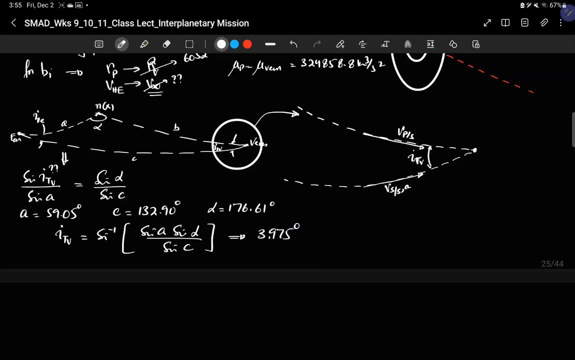 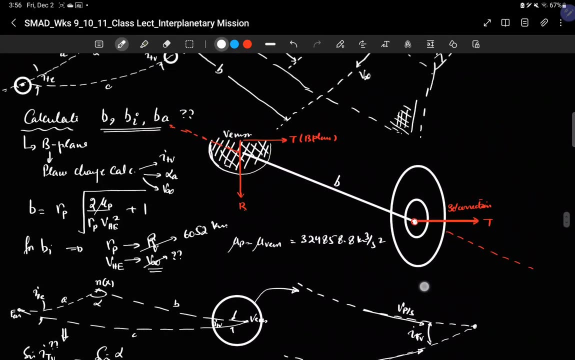 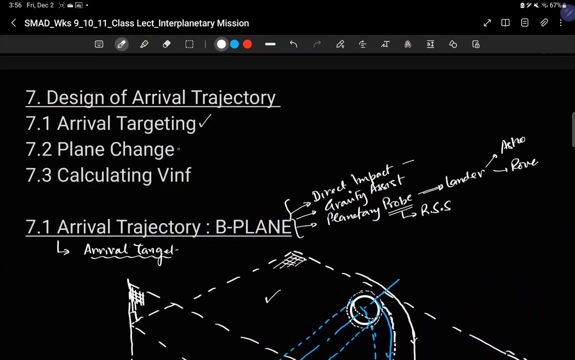 This is the inclination on the transfer trajectory that will be required to enter into the Venusian orbit. So this is our first step, which is determining the plane change and, as you see, so we had the arrival targeting and we are now solving for the plane change. now the next step to 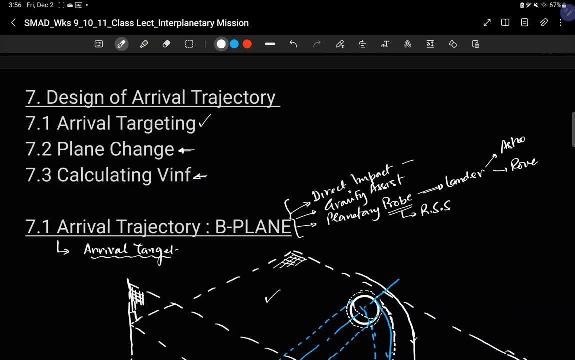 the plane change was to calculate the distance between the two corners the plane and at the V infinity, so that once we have these two parameters then we can go back and calculate the value of B, the value of B i and the value of B a, because to calculate the value of 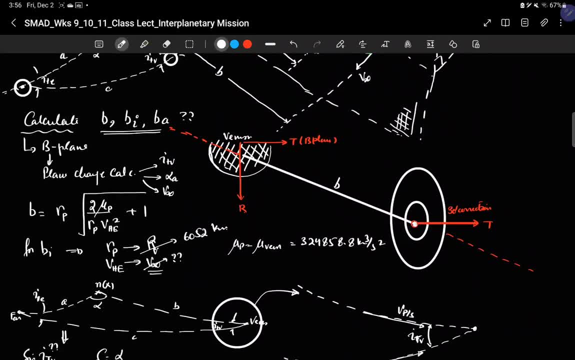 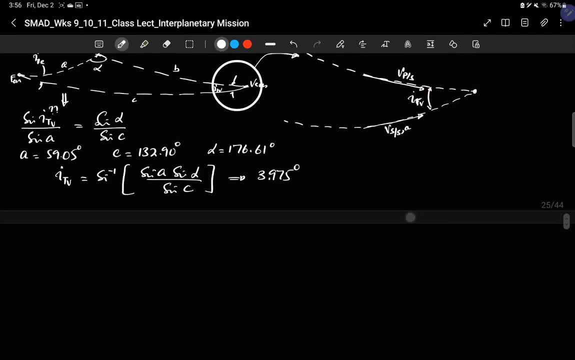 B, i, B, a. we need the value of V infinity. So to get the value of V infinity, so the V infinity square at arrival. and what can we use? We use the same kind of yes, the triangle, the velocity triangle that we did. 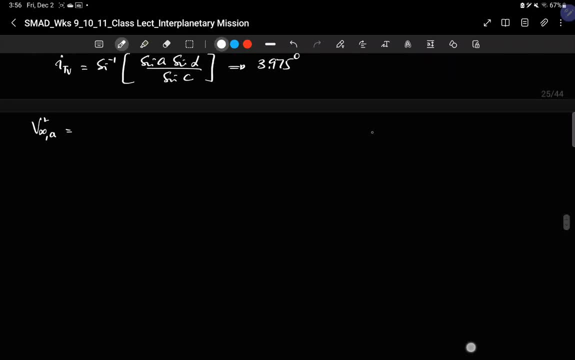 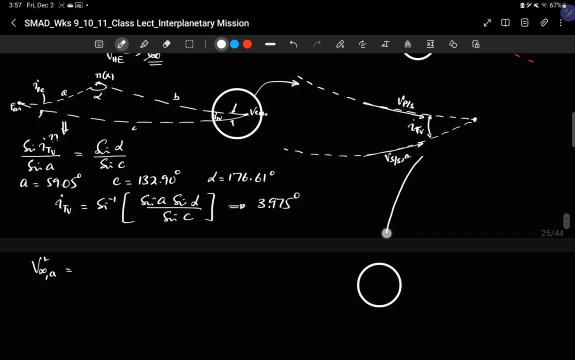 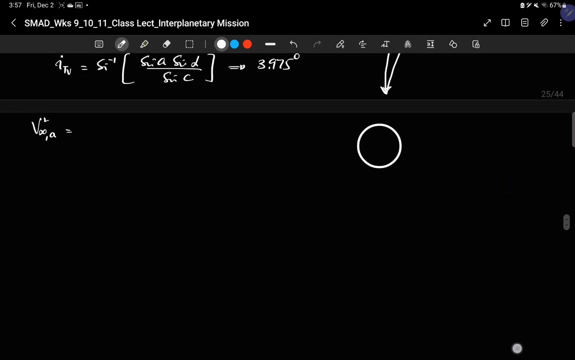 the last time. So what kind of velocity triangle will exist now? So this is Venus. So now I am actually expanding this figure. I am expanding this figure into a two-dimensional figure. So this is Venus here and the trajectory of Venus, for example. that is the trajectory. 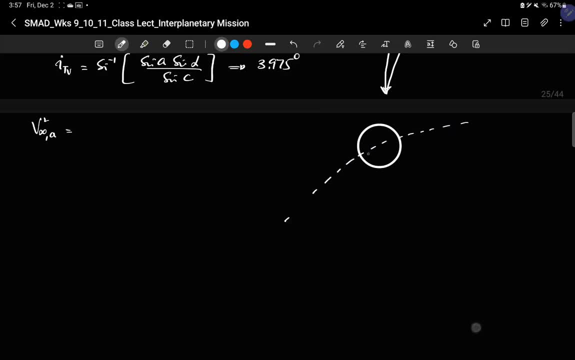 of Venus. So the local horizon Of the Venus is mapped here in this position. That is the. in fact, we do not need to put an arrow here, We just need to put a dotted line that is showing the local horizon of. 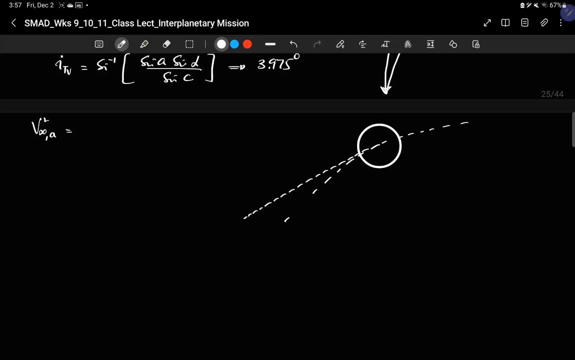 Venus, from which what was measured? The flight path angle. And if this, if the blue is the trajectory of Venus, this was the trajectory of Venus around the sun, then this would be the velocity And this would be the velocity of Venus V, of planet, with respect to sun. So this angle, 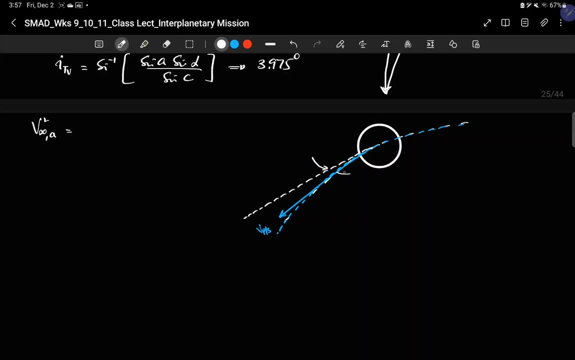 between the two would be the flight path angle. This here is the phi flight path angle of Venus with respect to its own local horizon, and it would be measured in the horizontal plane right. So I am drawing a horizontal plane here Now. 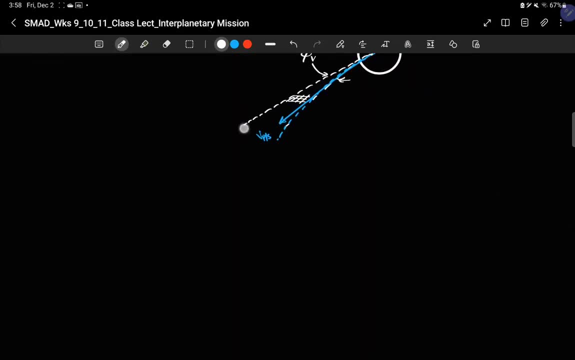 … ITV degrees below this plane. vertically below this plane is the position of the space craft which is coming in from around. so this space craft was coming in from behind and this would be the position of the space craft crossing underneath the planet and the angle would 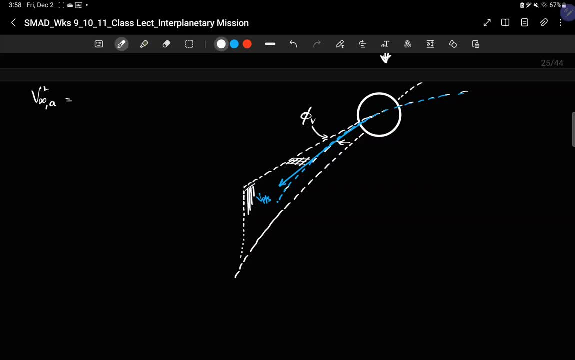 be now measured in a vertical plane. please refer back to the previous diagram. also, we did this in the last class as well. so this is a vertical plane and this vertical plane follows an angle which is ITV. so this is my IT of Venus, which the space craft is following. 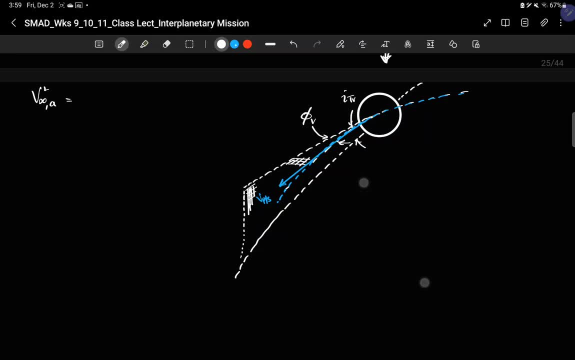 and then this space craft has a velocity vector, is following its own. so this velocity vector is with respect to the centre of the Venus, is, let us say, going outward, And this is in the lower plane. remember, this is in the lower plane with respect to the 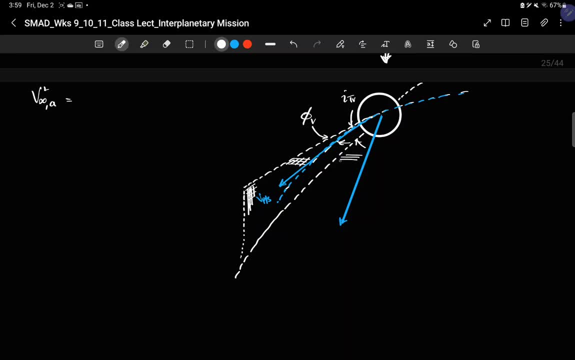 incoming. so this velocity vector is in the plane, in this plane. so we have two planes: the velocity vector of the space craft with respect to sun at its arrival, And so what did we have at that time? we would then take the V infinity. we would then take 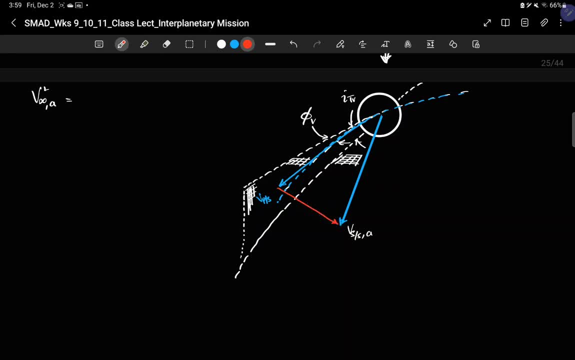 the vector connecting these two. so this would be your V infinity at arrival. and we had a slant angle and we have a slant angle between the two, so this slant angle would be your arrival alpha. so this slant angle is your arrival alpha and we can solve this slant. 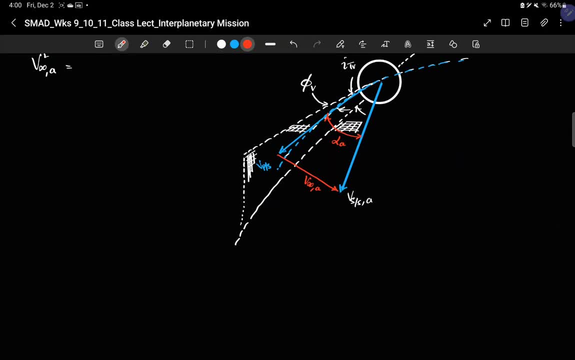 angle in a planar triangle. So the velocity vector of the triangle that they are forming is a planar triangle, and you have to get this thing developed for every single scenario. So now, if you take a two dimensional look of the vectors, then what do we have? we will 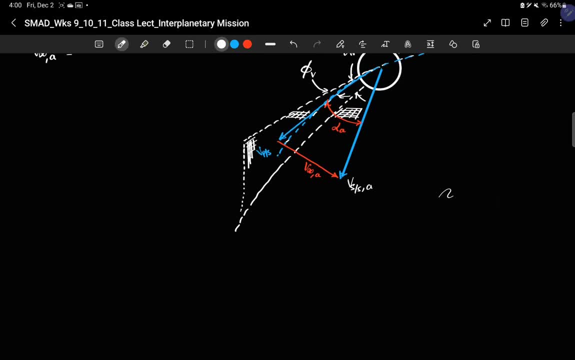 have at. this is Venus, for example, here the position of Venus, and there is a flight path angle, phi. So, since we want to get something like three dimensional volume concept, that is what is done, so for this i will write 3 times 5 v. so this is 5 v and this is the velocity vector. 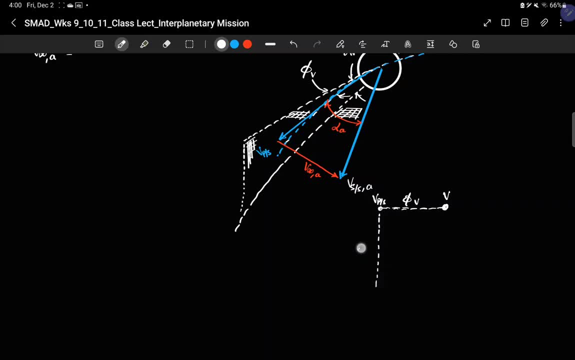 of. so this is velocity vector of the planet with respect to sun coming out of the plane of this paper And below this, at an angular position, at distance i t v is the plane of the space craft which is at a certain distance, so that is angularly measured as phi. 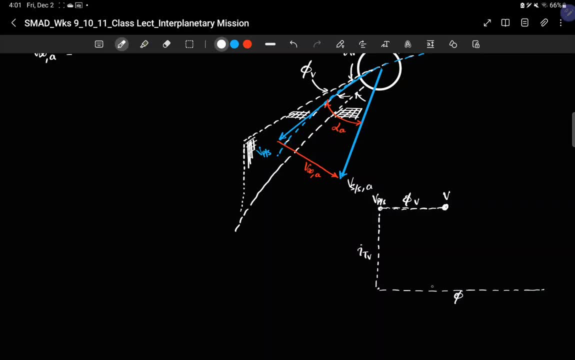 So that is the distance within the whole group. If you have seen the sender of comet at a particular distance, we will observe some instructions. so that was once we calculated the stress ofiesz trying to do log結weeding of the spacecraft. so we usually refer to this as I forgot to mention this figure. 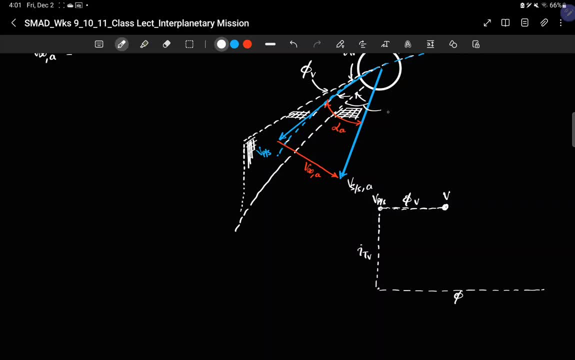 so this in this plane is your phi. this is the phi of the spacecraft which is at arrival. so therefore this phi is the flight path angle of the satellite. so we call this flight path angle of the spacecraft on the transfer trajectory, at the arrival. 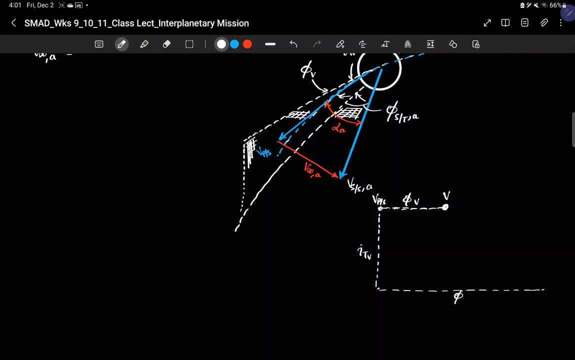 This is exactly how we mentioned the last time. also fly of the spacecraft on the transfer trajectory at the departure. so this is S on the transfer trajectory at arrival. so that is the angle This means. so this is the angle phi, from here to here is your ITV. 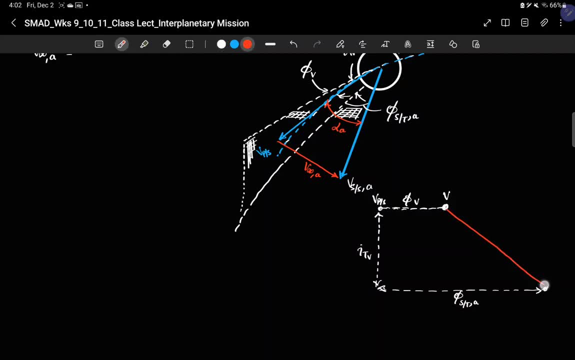 so that leaves the red. if you connect these two points here, then, and not to forget that this was your velocity of the spacecraft with respect to sun, So this is your velocity of the spacecraft at the arrival, so this will be your V infinity. 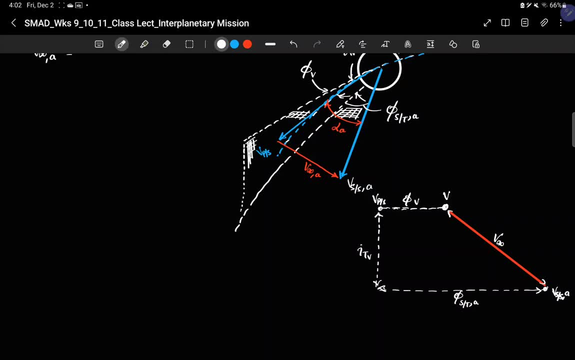 between these two points. so this is your V infinity, and the angle corresponding to the slant angle corresponding to this V infinity is your alpha at the arrival. So this is exactly how we constructed the departure triangle as well, except for the fact that there was 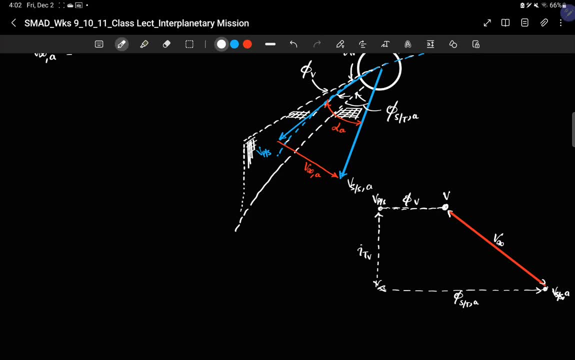 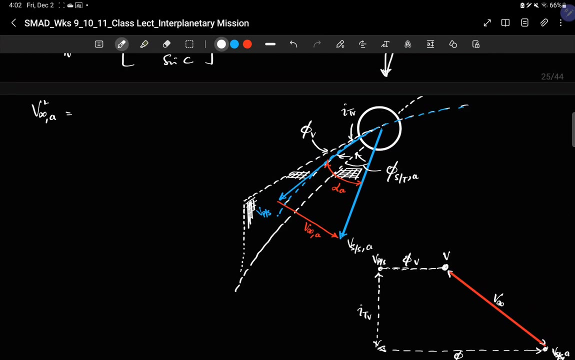 a difference between how the angles were measured depending on the position of the earth, because the angle is outer to the venus and the venus is inner to the earth, so the direction is on both. the angles are measured from the same side. So V, infinity square A, we use the triangle. let say we call this triangle center of the. 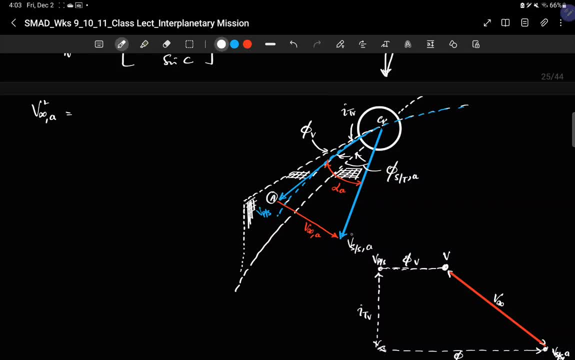 venus and A here and B. So if we solve triangle CV, A and B. So what happens is that it is right if we to the right, So if we are right, it is. So we can get the value by the simple planar cosine rule, which will be V, infinity square. 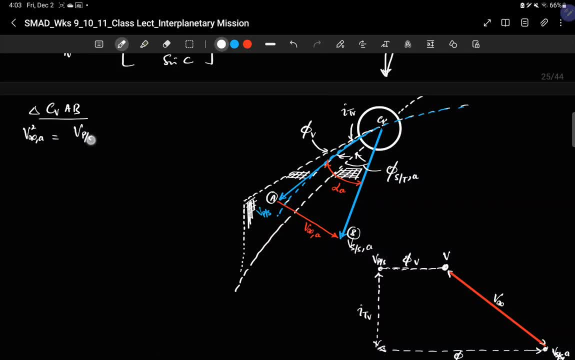 at arrival will be equal to velocity of the planet respect to sun square plus the velocity of the space craft with respect to sun at arrival square, minus 2 V, PS, V, S, S A. into cos of which angle Included angle is alpha a. so into cos of alpha a. 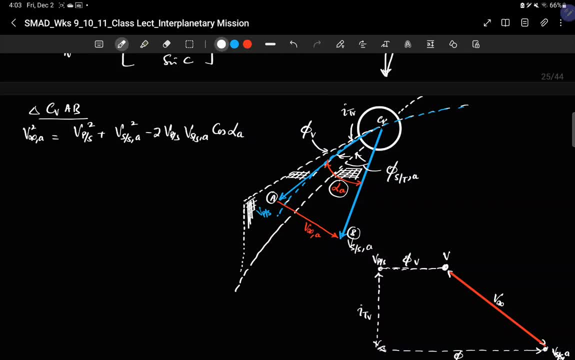 So now we also to get the angle alpha a. this triangle was used last time. so we do not know this thing, but we do know the V PS, the velocity of the planet with respect to sun, in the beginning, in step number one, when we were doing the planetary calculations. so at that time 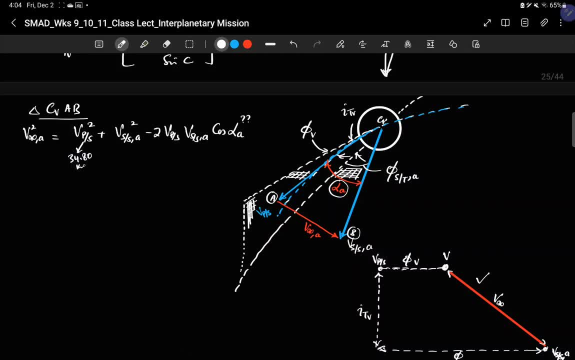 we calculated this to be 34.80 kilometers per second. the velocity of the spacecraft with respect to the sun at the arrival we did the last time was 37.57 kilometers per second. so all these value, but what we don't know is this value. so, as a result, we don't know this alpha as well. so what? 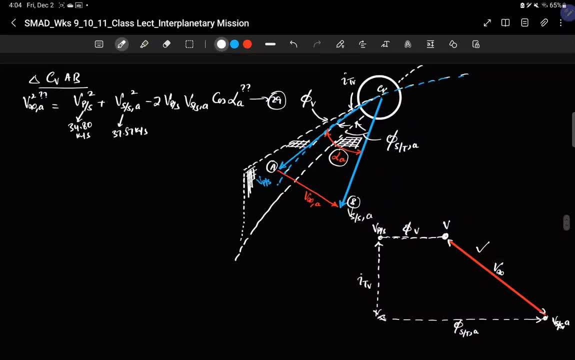 we can do is we can just put this as 29, so we can use the equation for this here to determine what is the angle. and the equation we used was cos of alpha a, was actually cos of itv into cos and now, because this alpha a relies on the difference between these two angles, so it relies on this. 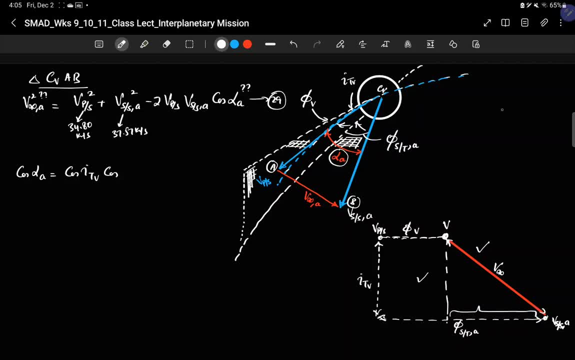 side, the previous k instead of the previous k. the previous k, when we were departing, we had alpha on this side, we had this on this side. so the angle was based on the sum of both the angles, isn't it? but here it now relies on the difference between the. 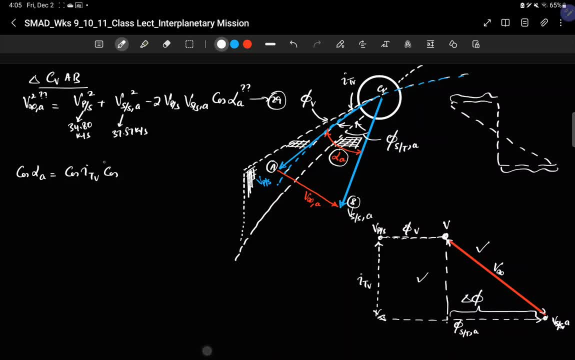 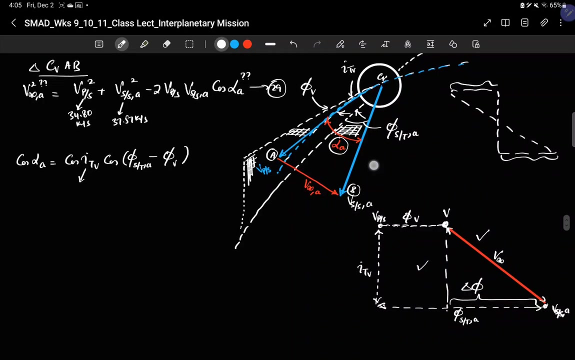 delta phi's. so therefore that will be the cause of phi, of the spacecrafts at on the transfer trajectory, at arrival: a spacecraft on the transfer trajectory at arrival, minus the phi of the phenester, plus the rebuilding центр at the personalities of eachThank you very much. Thank you very much and see you tomorrow at 9rac. 0. dry off the venus on its own wind working. Now we know these values by. we know the value of itv. we calculated the. yeah, we know the value of itv. we also know the value of. we also know the value aphrystia relationship, because 3.9407, and we know the fly path angle of v, all calculated in the previous h switch. UE Harvard. dean of Toy들 of a And familiar to the freedom of to be. 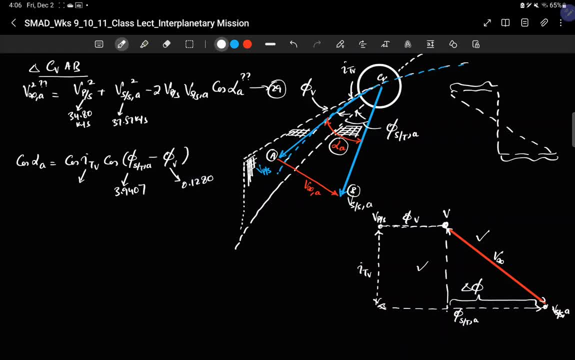 previous steps, 0.18280, and this is this was 4.455.. So the alpha A would then come out to be about 5.509 degrees. Now, once you have the value of alpha A, the V infinity. now. 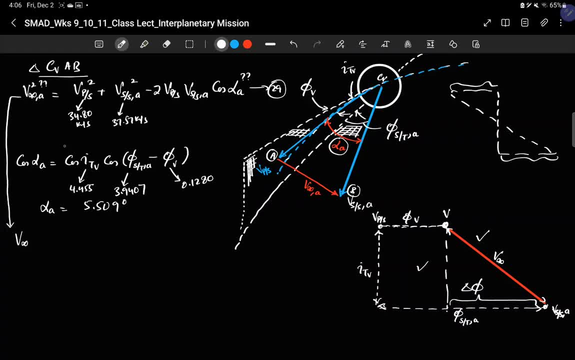 we can put this value of alpha A back into this relation here, So it goes back right here. So that would mean that your V infinity would come out to be 4.442 kilometers per second. Okay, Once we have the value of V infinity and 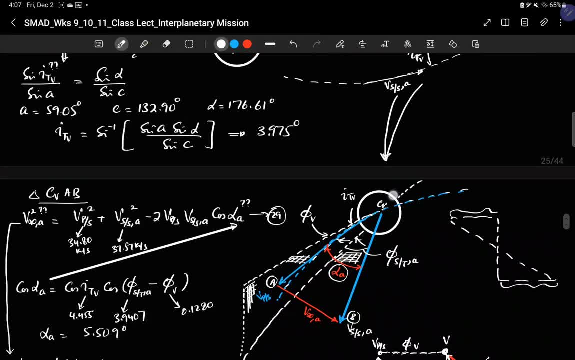 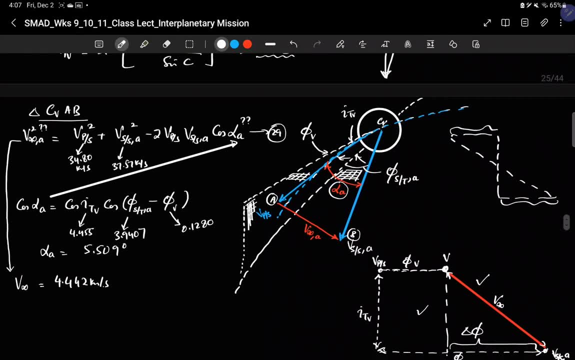 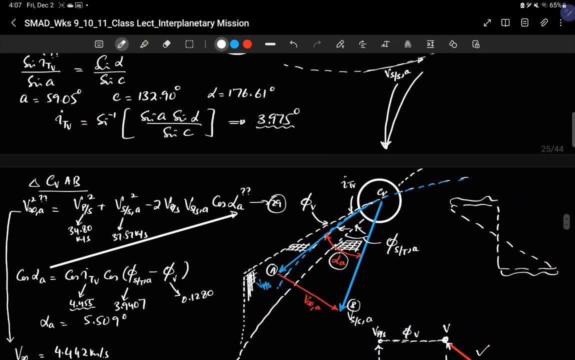 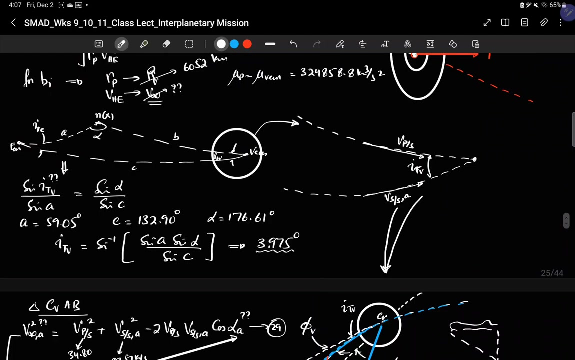 This. you may ask that you get a calculation of 3.975 here and instead of 4.455, it is because these two calculations were performed on two different ephemerides. So if you follow the previous ephemeride then you will get a 4.455 right here. Okay, That is the only. 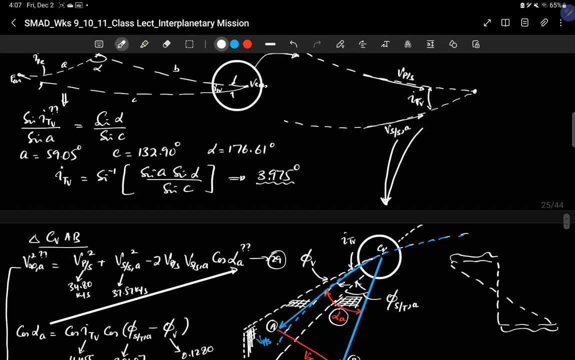 reason. So you could always ask this question. So I have answered this. because I am I will be unable to do it, So I have to go back to the previous slide. But all along I was calculating at two different ephemerides, just checking the difference between the two results. 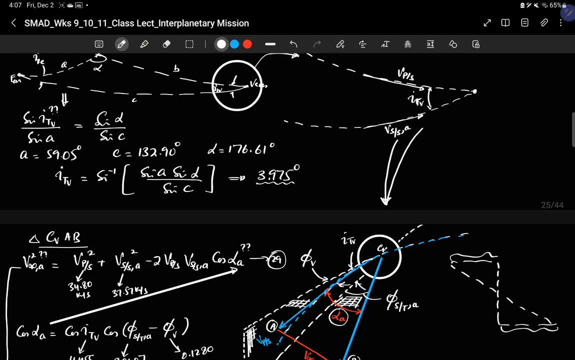 Okay. So there is a small hunt of 0.5 degrees that occurs between on a day to day basis. If you change the day, so it will cause the change here. Okay. So this- this should also go to. 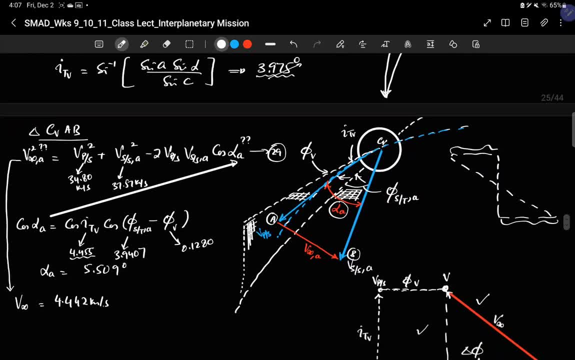 So you cannot use this one. So you can use this one, No problem. It will just create a very small variation here, But since we are following, the previous calculations were based on 4.4551.. This depends on the. 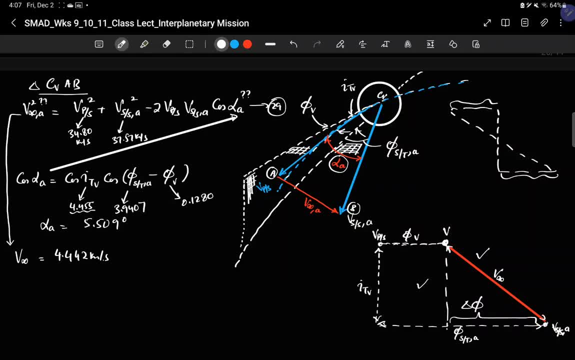 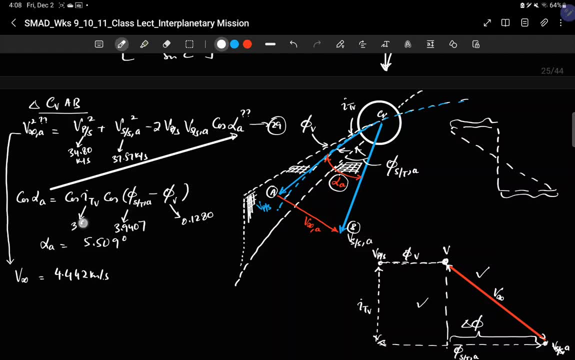 time management. You see, this is here, So this is here. This is basically the start point. So here we are. See, this is the start point. Here we have actually two. There are some 4.455, i guess. so sorry, that was the itev, my bad, that was it of the earth. so this is 3.975, okay. 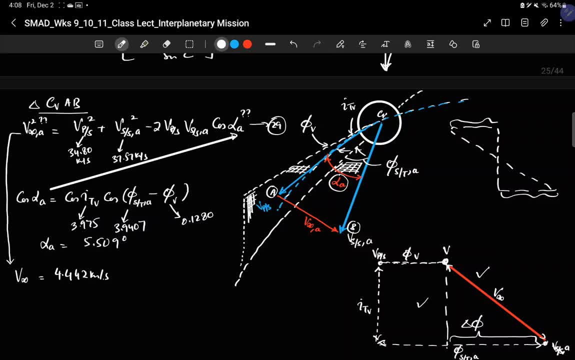 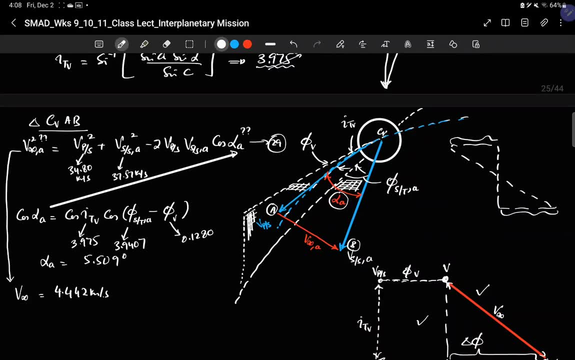 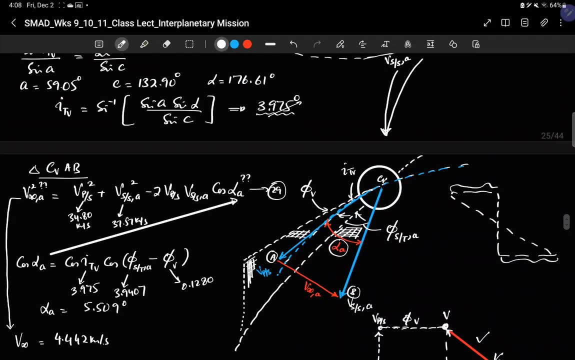 okay, i don't know this is correct. this is calculated with alpha a, 7 to 3.9. so my bad of writing that 4.5. i forgot those numbers. there were so many angles, i forgot the numbers for that angles. okay, the only thing is that sometimes you may get a small variation of 3.975 maybe. 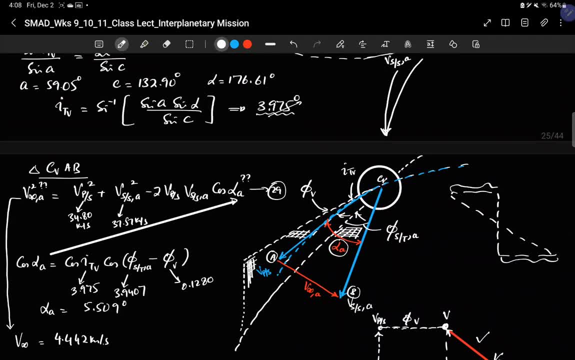 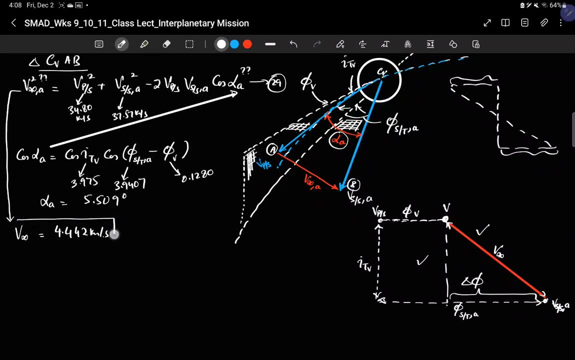 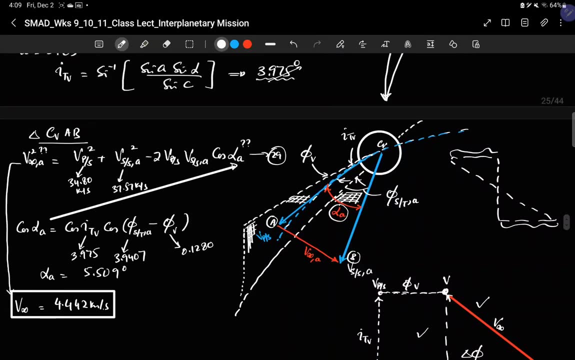 become 3.98 or 3.976, so don't get worried about that part, okay. okay, v infinity is done. we have a very important figure. this is the uh. this is the infinite velocity now available to your spacecraft on its arrival, and we also know the value of alpha a. this is another important angle. 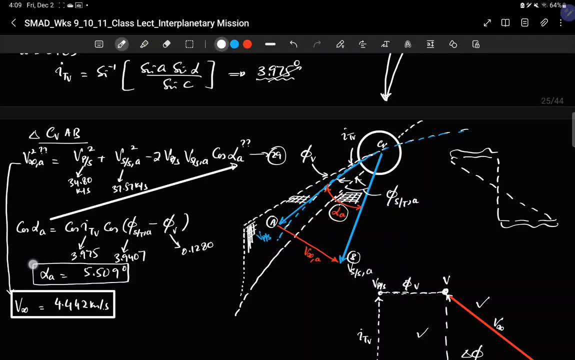 because this angle will determine how, the how with respect to the position of its previous, because this is past conic. so you have alpha a with which the spacecraft is going to approach at the sphere of influence. this is the alpha a with which the spacecraft is approaching at the 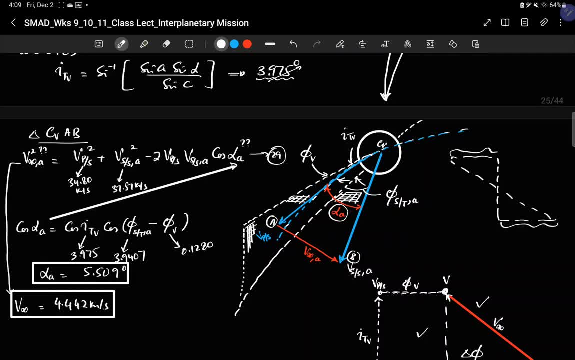 sphere of influence and will be looking, uh at the at the planet for approach. this is yes, with respect to that planet's position. this is how it's going to look at the angle and we're going to draw that triangle. they're going to specific triangles for that. 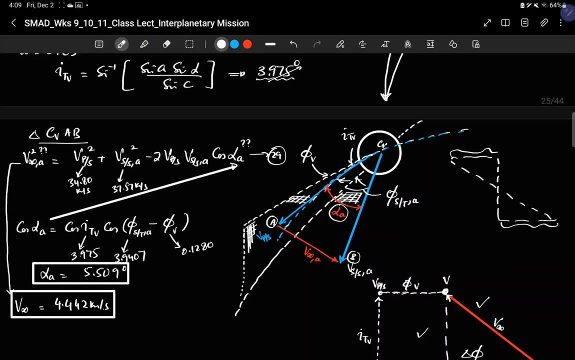 so the velocity is, in this case, more than the hyperbolic excess, because we are only, uh, having a very small velocity at the very end. so are we? is there any contribution of the planet's motion, exactly because you have moved inwards. this is an, this is an inner planet. so the moment it is just like 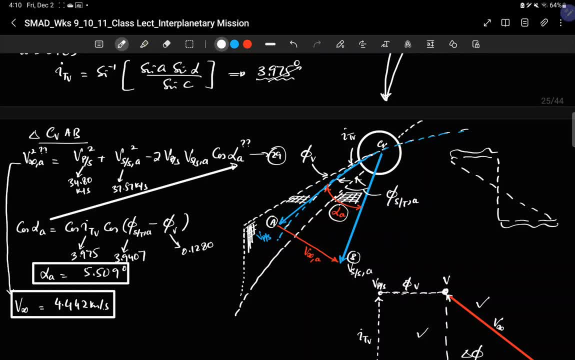 going, coming closer to the earth. so the moment you are going from outer planet to the inner planet, your velocity will increase. if you are going to an outer planet like mars, the v infinity would be less than your hyperbolic excess velocity at that time. so this v infinity, this is the velocity which is going to fall onto the planet.